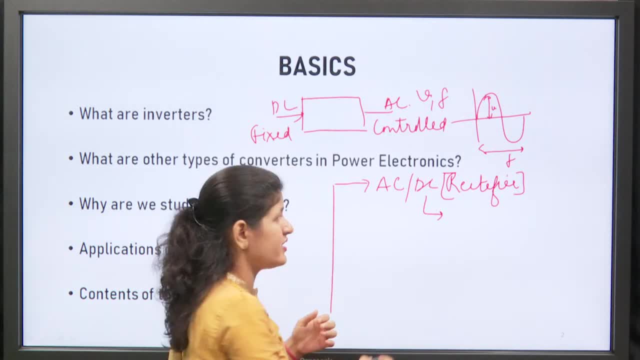 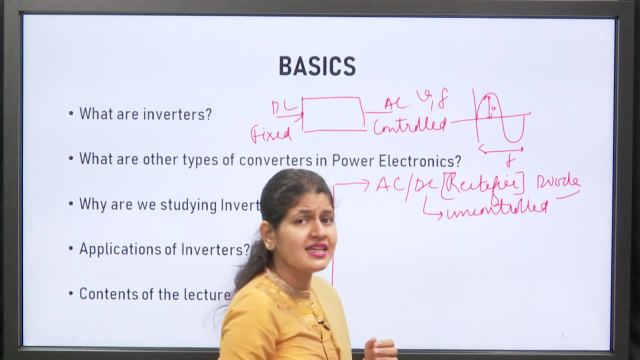 this DC is uncontrolled DC. Uncontrolled DC means we cannot control it. Why? Because the AC to DC rectifier uses diodes, And diode's by themselves is an uncontrolled device. and why is this called a uncontrolled rectifier? Further in power electronics, we have studied 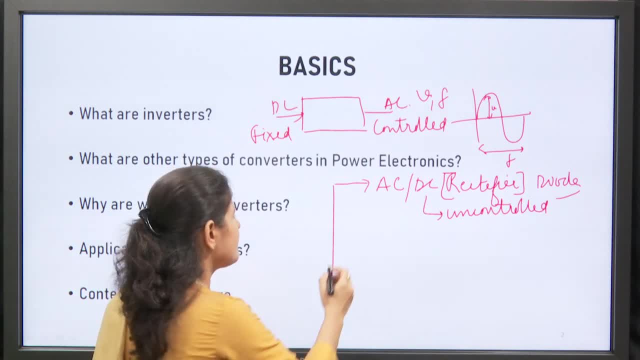 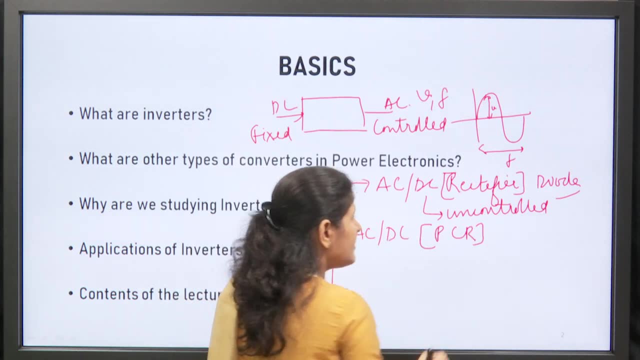 similar AC c нуж DC converters Next in power, likeIntronics, AthleticsCenter, 요� orin electronics. we have seen AC to DC converters, which we call face controlled rectifier. What is the difference in these two devices? The device Salutment we use in face controlled. 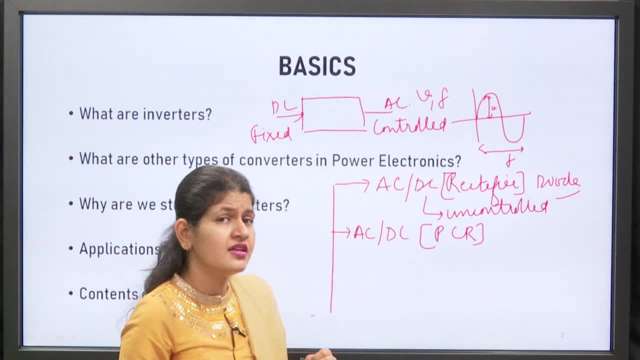 rectifier is known as thyristor, We call the device thyristor, which is very easily grabbed in a thyristor or thyristor family. So the fine hired device which purifies the circuit gets and thats the direct unit. We say this orに conducting other shoulder. Conversely, we 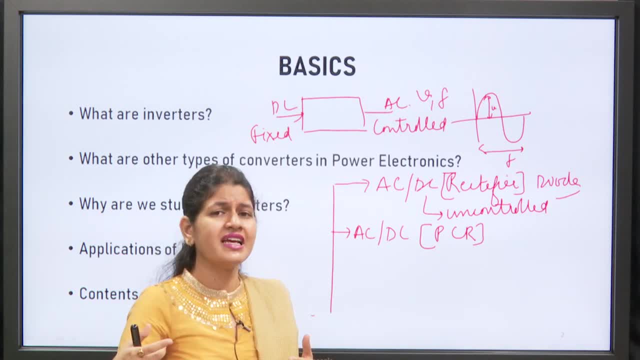 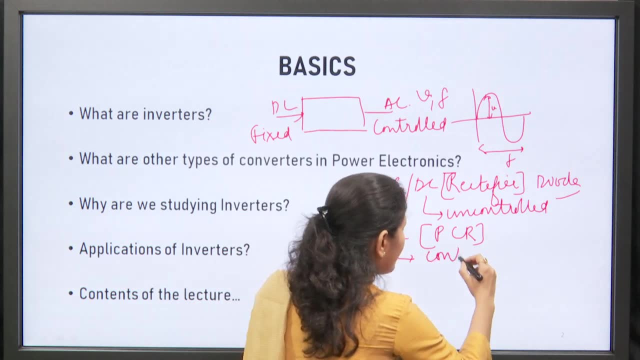 thyristor family ka koi bhi element To ye jo thyristor family ke elements hai. ye apne aapme control devices hai. Isliye, ye jo DC hume yaha milti hai, wo milti hai hume control. 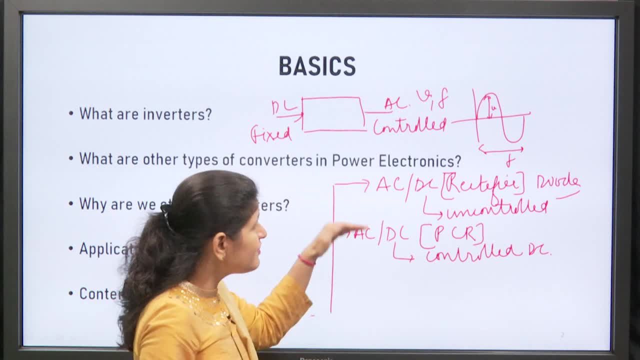 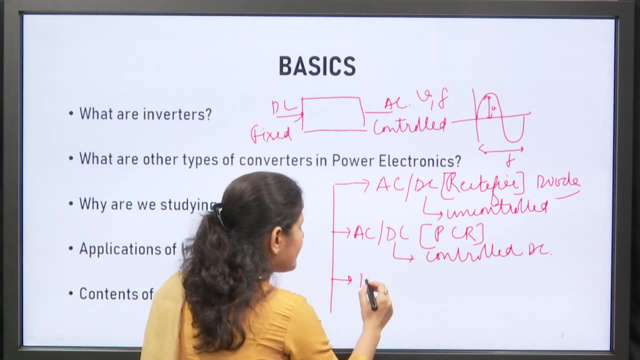 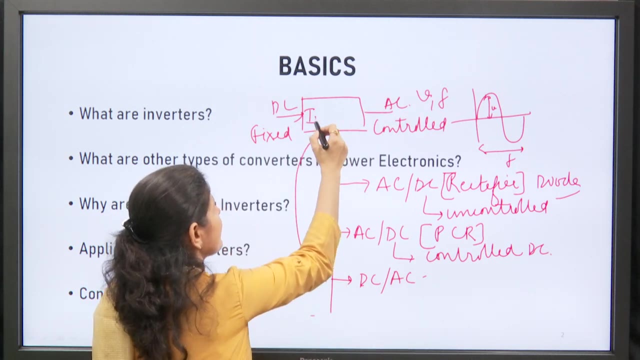 DC Control, DC Thika To ye difference hai basically rectifier, ya diode rectifier, or phase control rectifier. me Jo third type ka configuration hum padte hai, wo hai DC to AC converter, Jise hum inverter kaite hai, Aur yahi inverter aaj hum discuss kar rahe. 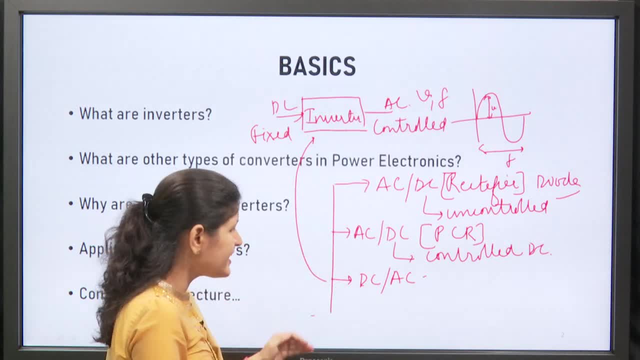 hain Thika Yahi inverter. aaj hum discuss karenge Iske alaaba further. ek aur classification rahe jaata hai: wo hai AC to AC type ke converters? Aap dekh raha hai, ki sabhi combinations use. 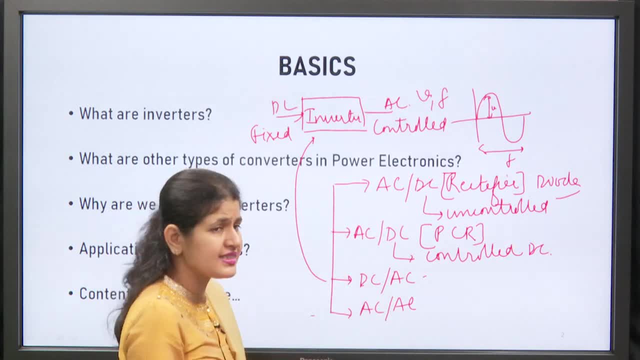 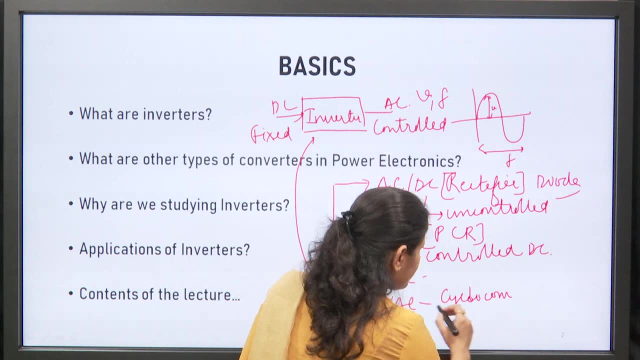 ho gaya hai: AC to DC, DC to AC, AC to AC, Thika AC to AC. me ek hai cyclo converter, cyclo converter, aur dusra hota hai AC voltage regulator, AC voltage regulator, Thika To. 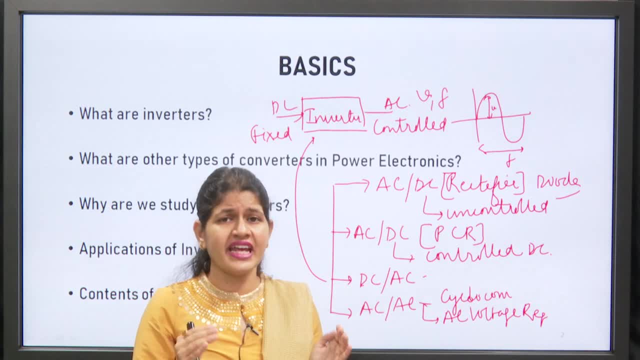 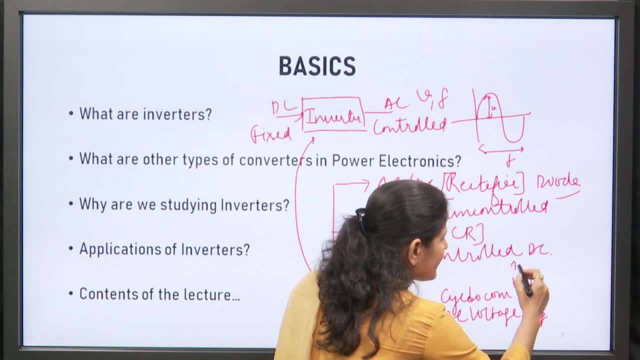 cyclo converter aur cyclo converter Aur AC voltage regulator. Ye dono hi AC to AC converters hai, Lekin dono me difference ye hai ki cyclo converter me voltage of frequency maan lete hai, ki ye input ki hai To jo output. 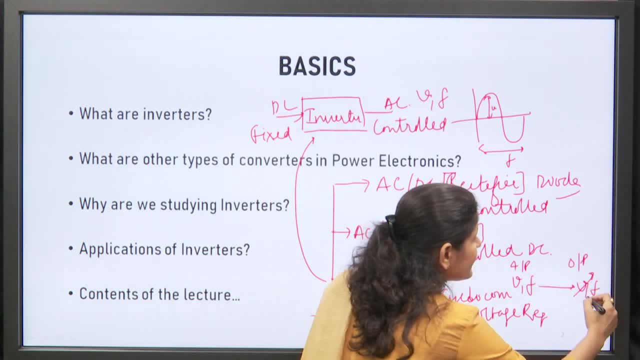 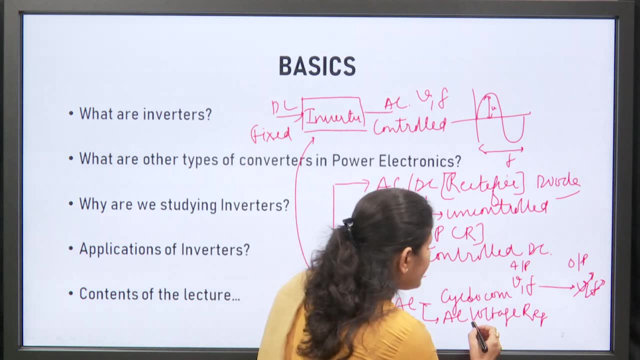 ki voltage of frequency hai, wo dono hi hum regulate ya control kar sakte hai. Thika Output ki voltage of frequency dono hi controllable hoti hai. Japki in case of AC voltage controller, voltage of frequency agar ye input ki hai to isme output voltage to vary karte hai To. 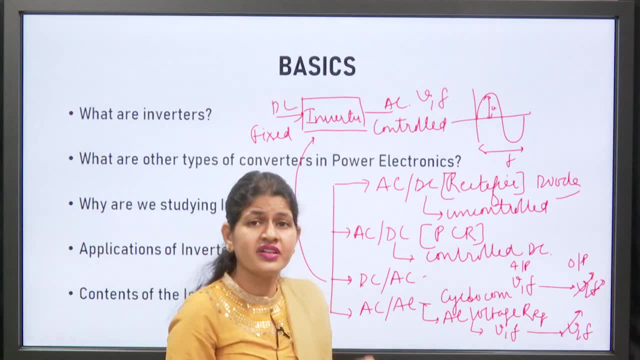 isme karte hai, Lekin output frequency is same as that of input frequency. Thika Iske ala wa ek aur type ka converter rahe gaya hai, Jaisa ki aap dekh bhi rahe ki ek combination aur. 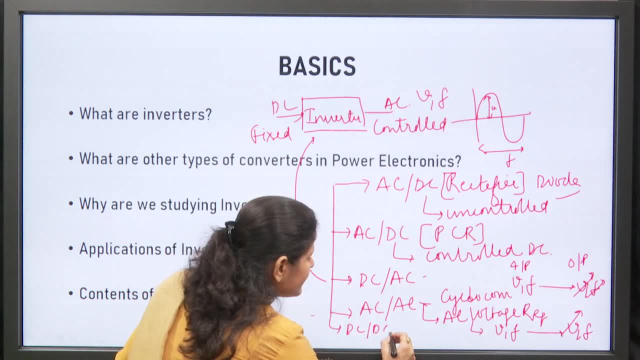 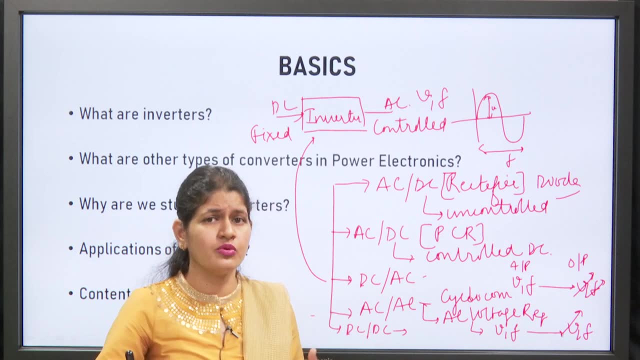 rahe gaya hai, Wo hai DC to DC converter. Thika DC to DC converters, jene hum choppers naam se padhate hai, Aur chopper ke baad further usse buck converter, boost converter ya buck boost configurations me padhate hai. Thika To ye itne tarike ke power electronic converters. 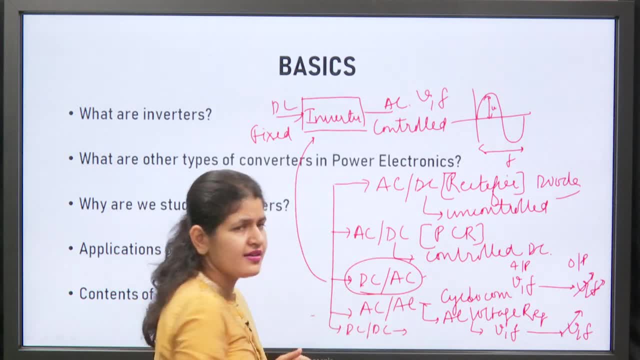 hum waise jaante hai, jen mese. ye hamara main focus hai. Aap dusra point hai ki hum ye padhate. kyun hai Inverters padhne ki zarurat kya hai Hamare gharon me? jo bhi AC supply aari hai, 230 sin, omega t, jo bhi AC supply aari hai usme hamari. 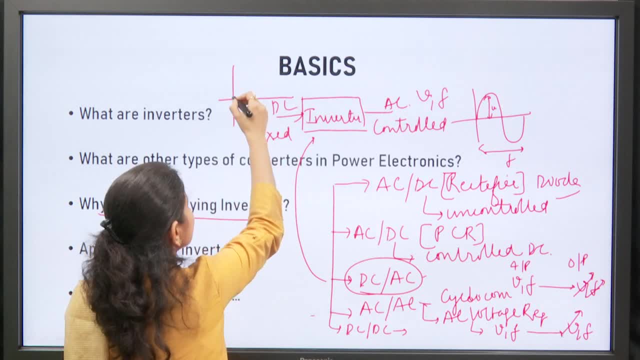 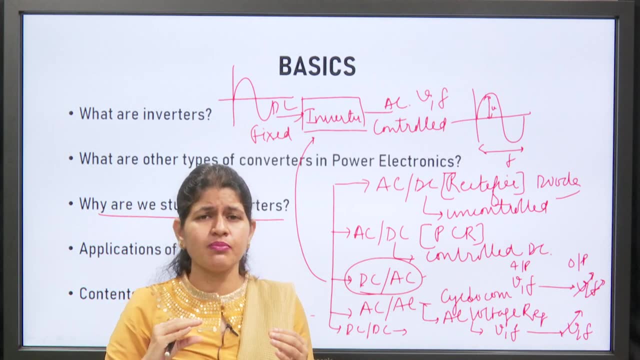 requirement. kya hai Jitni zyada clean, jitni zyada clean AC supply aayegi utna zyada hamare le better hai load end pe jo consumers hai Kyuki agar AC supply me zyada fluctuations. 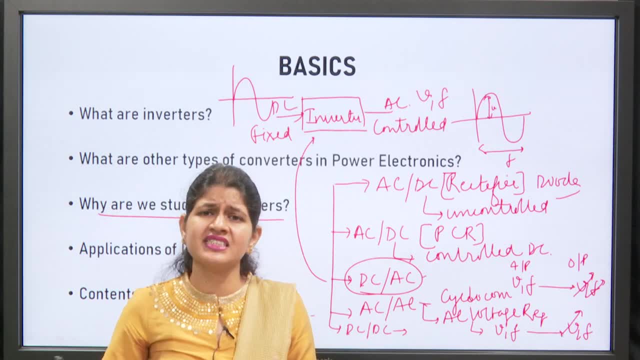 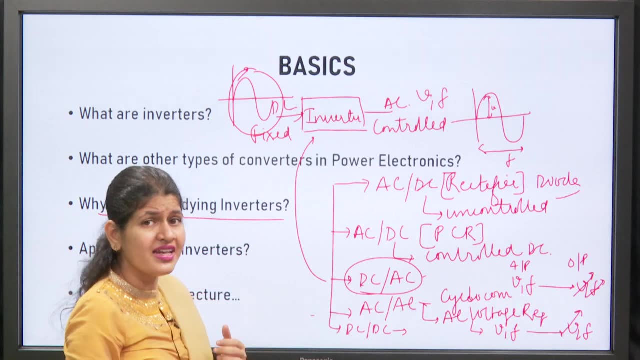 huwe ya zyada harmonics huwe to wo hamare hi ghar me use hone wale several equipments ko destroy karenge. Thika tech to ye inverter. kya output jo hai. AC pure wave form aana is very important Aur. 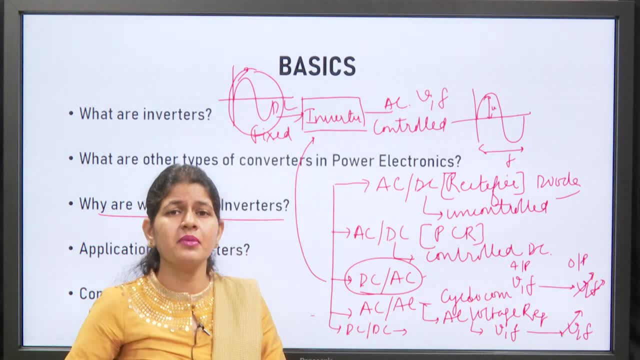 ye kum kab la payenge, ham kabb ye jaan payenge ki AC, jo hamier mel rahi. eh boh hume pure cyanoit also milein, Jab hum us inverter circuit. a detailed analysis, ya, details study. 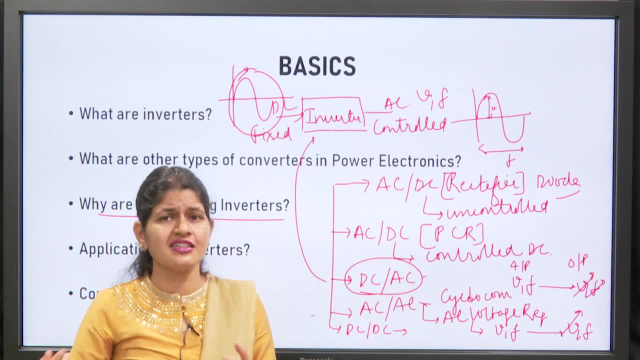 karenge ham yuya janenge ki wo alag alag loads pe alag alag tarike se kaiser respond karta: hai yase resistive load, hai aani bulb load hai usme inverter. kaiser respond kara. hai RL load hai fan load hai inductive load pe kaise respond karta hai to alag alag loads pe kaiser respond karta hai To alag alag loads pe kaiser respond karta hai: espe Ashwari es datare. 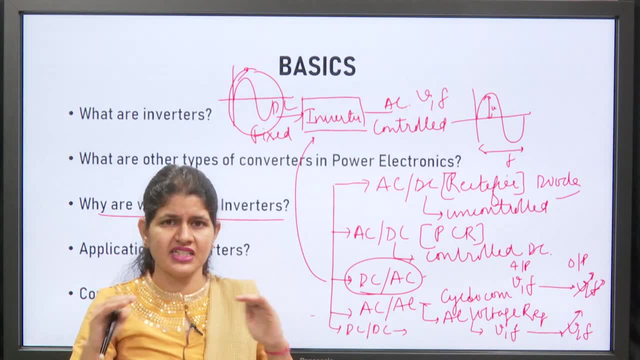 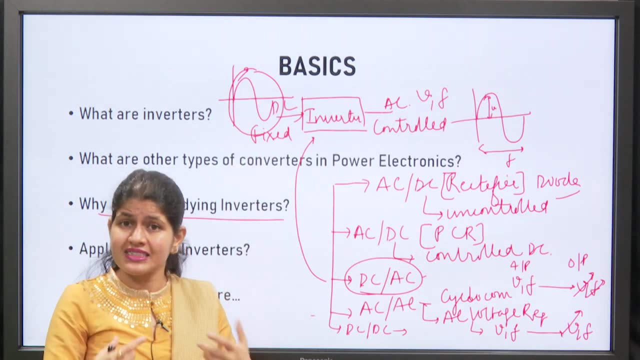 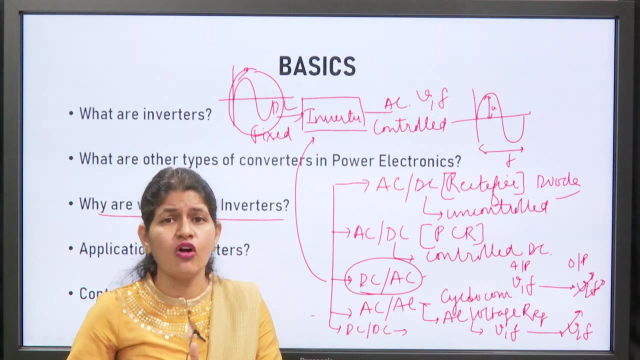 So, according to different parameters or different loads, until we do not know the configuration or the response of the inverter, how will we bring this pure AC sinusoidal, how will we be able to decide that which control strategy should be applied so that the pure AC sinusoidal 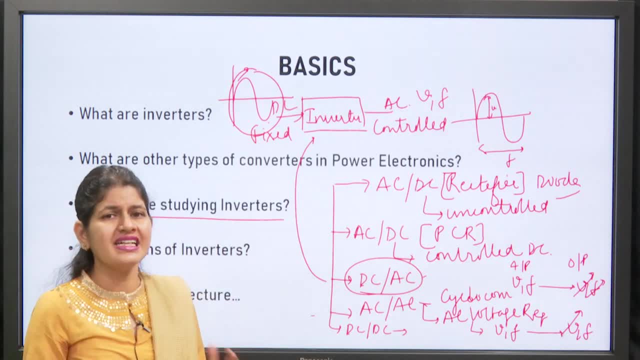 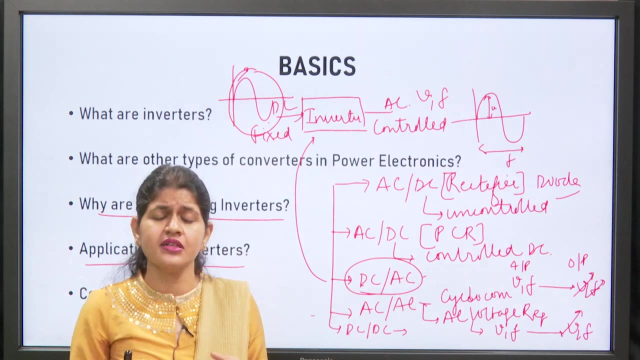 that has to come on the output of the inverter. for this it is important to read the inverters in detail as an electrical engineer, Which is application of inverter. So in application, the most day to day application around us is the inverter used in our homes. 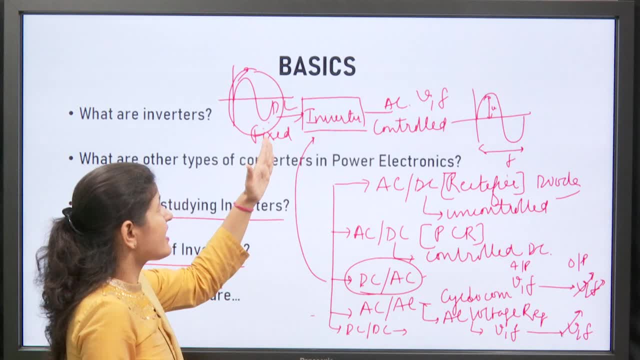 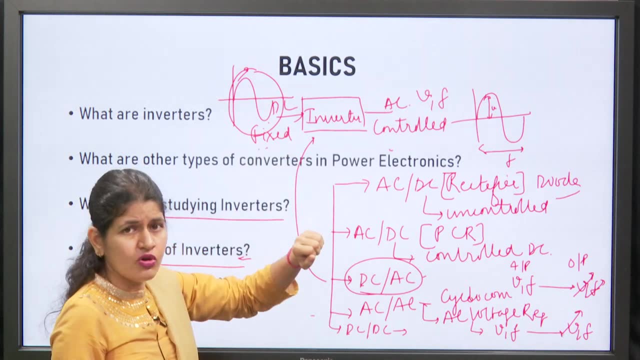 The inverters used in our homes. the inverter always remains DC fixed to AC controlled, that is, the output is controlled AC or variable AC and the input is always DC fixed. So the inverters used in the homes, what is used in place of DC source? 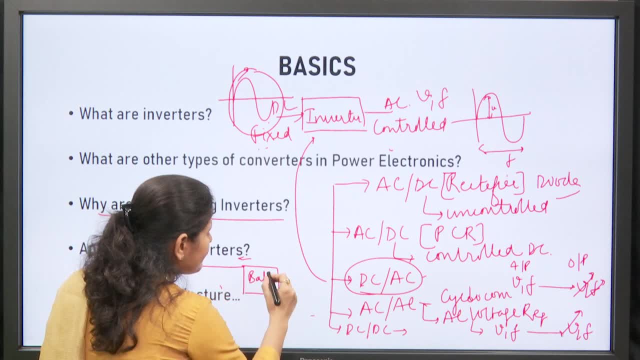 The battery is used in place of DC source. Ok, The battery is used in place of DC source. This battery works like a DC source. Then in the inverter used in the homes, the circuitry of the inverter is used in the. 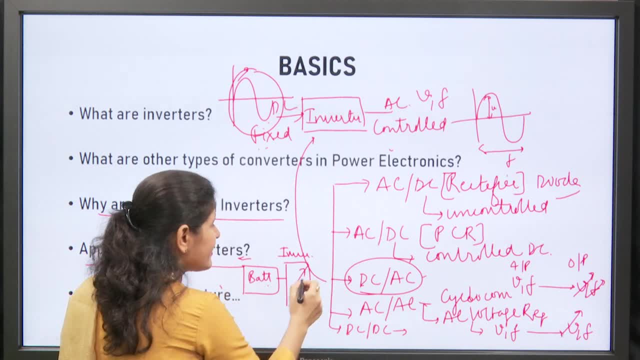 middle. We will read the circuitry of this inverter in this unit. whatever we are reading ahead, And the output of this is pure AC. This is the pure AC, or whatever our required or desired pure AC is, this is the AC that. 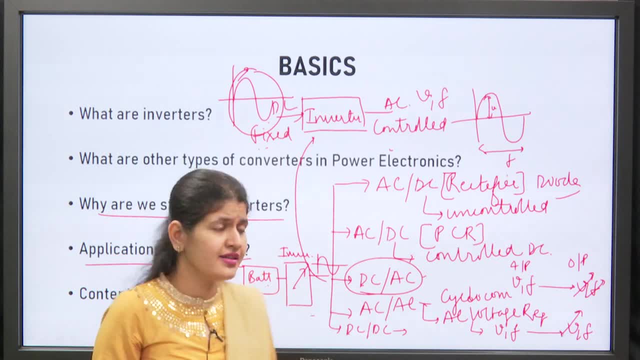 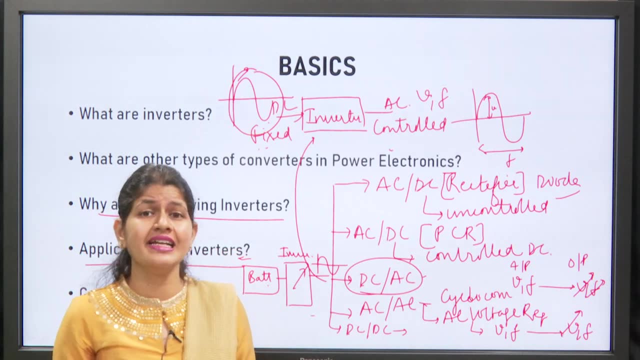 comes to our homes whenever there is no electricity. Ok, So this is the basic inverter used in the home. This is the basic inverter. Apart from this, there is one more application which is widely used in industries, that is, adjustable speed drives. 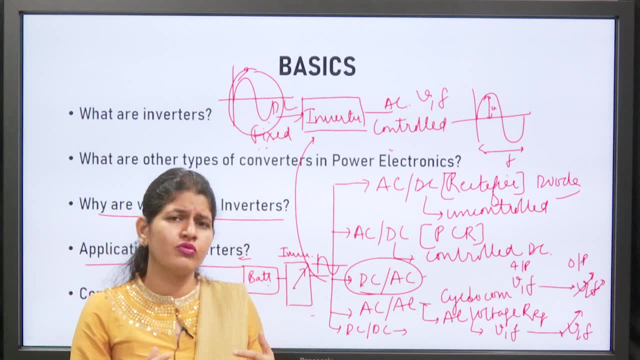 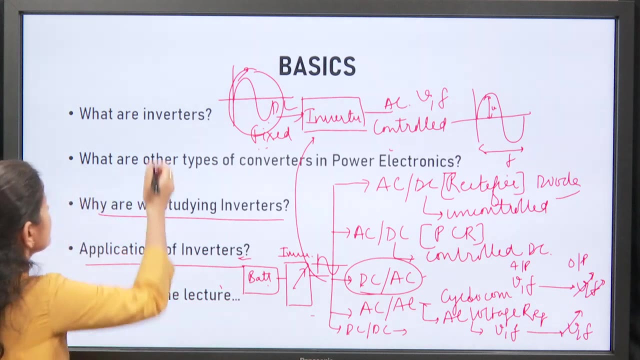 Before adjustable speed drives, induction motor and synchronous motor had some limited applications. Or anyway, induction machine is the most used machine in the industry, But still it had some limited applications. But with the help of these inverters, any machine, any AC is there. 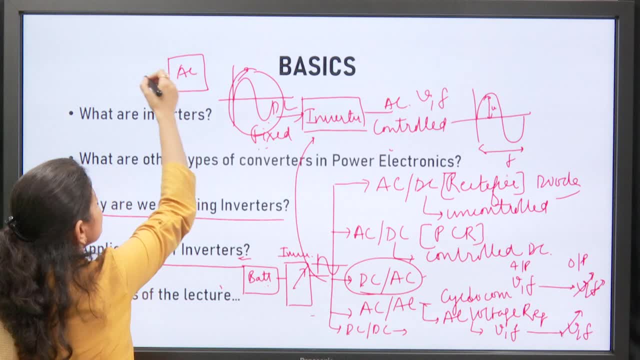 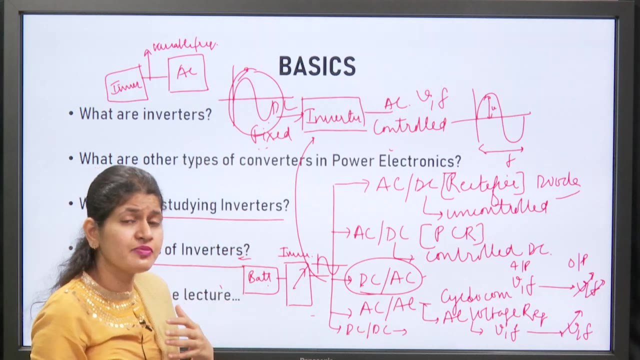 Ok, Any AC machine is there. If we put an inverter on the input of this AC machine, then the output of the inverter will be the variable frequency. Right, It can give the variable frequency. And in adjustable speed drives or variable speed drives, what do we need? 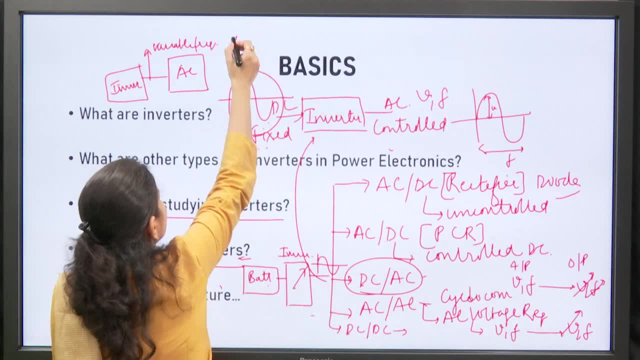 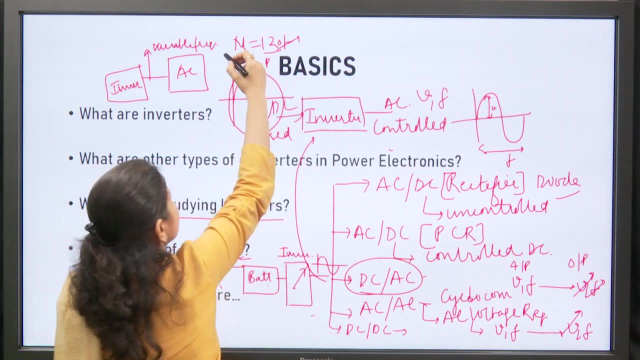 We need variable speed. So n is equal to 120 f by p. Ok, So if we can vary this frequency, then we can vary this speed also. We can increase the speed also. We can increase the speed also, Ok. 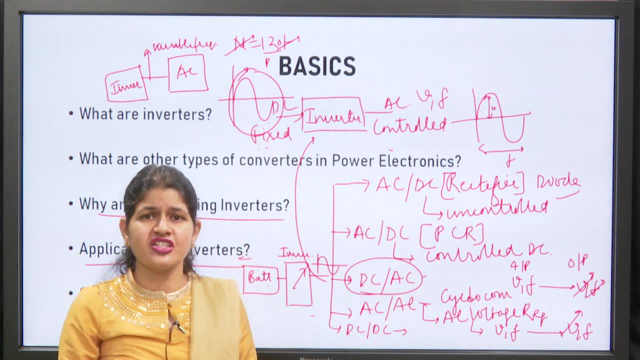 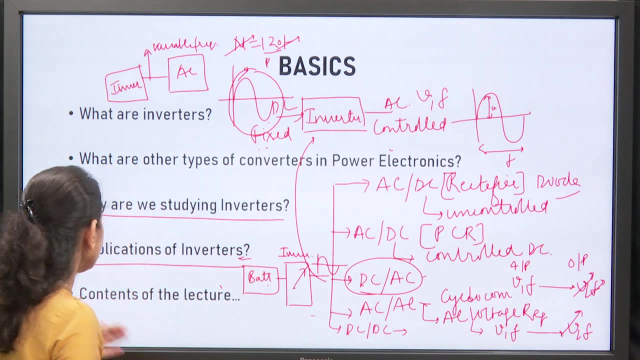 So, with the help of these inverters in industry induction machines, synchronous, their applications have increased more. Their applications have become more wide. Ok, This is one more example of this. Now we will talk about what we will further study in this content. 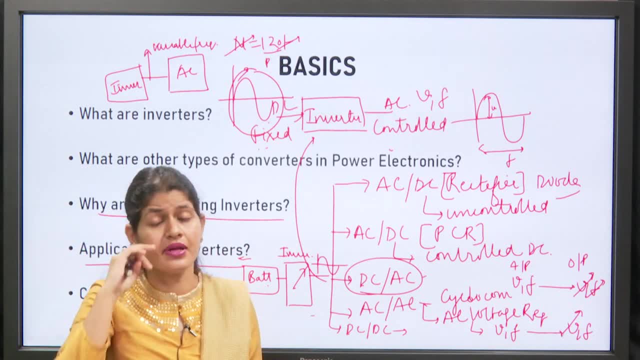 What we will further study in the lecture which we are taking right now. First of all, we will know that how many different types of inverters are there, Configuration wise also, And how they are classified broadly Further, how they respond with different loads. 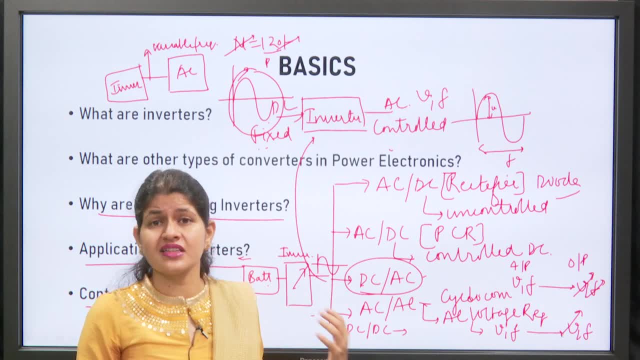 And apart from this, which commutation circuits can be used in such inverters? Commutation is to turn off the circuit. That means how can we stop the working of the inverter? One commutation. And apart from this, we will see different: single phase, three phase, different configurations. 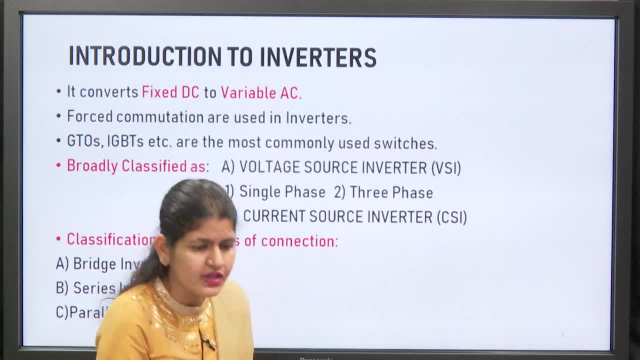 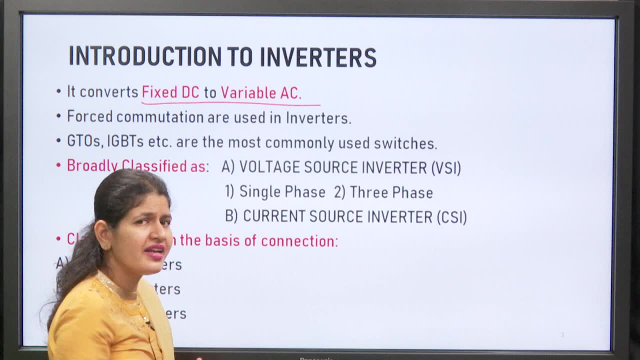 in this. Ok, Next slide. Next is introduction to inverters. So in introduction to inverters, we will see this thing. We will consider different types of inverters. So in introduction to inverters, In the case of converters, we know that it is fixed DC to variable AC. we also know what. 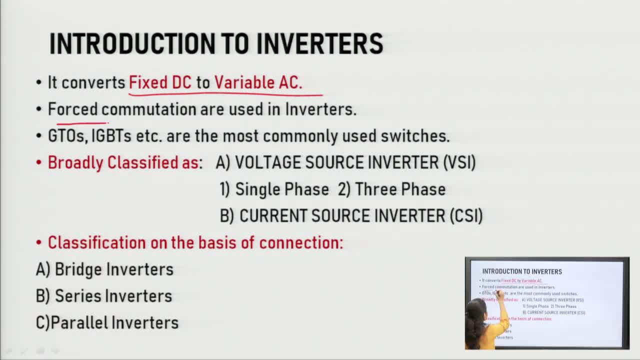 variable AC means. Next, we know what type of commutation is used in it. so we can see that we use force commutation In commutation, basically what we already know in different types of commutations. the first commutation that we read was line commutation. 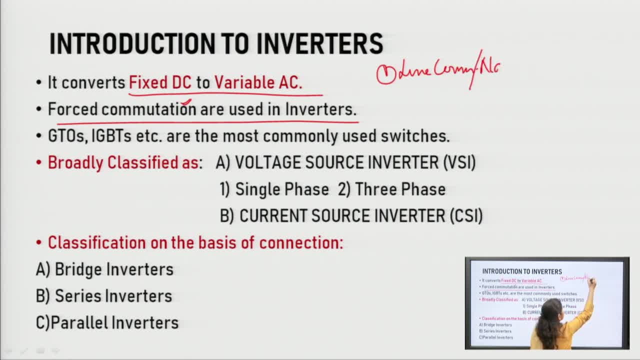 Line commutation is called natural commutation. Why is it called line commutation? Because the AC cycle. if there is a sinusoidal AC waveform in the input and this is the switch in the inverter- sorry, any switch where there is AC supply- then what is the property? 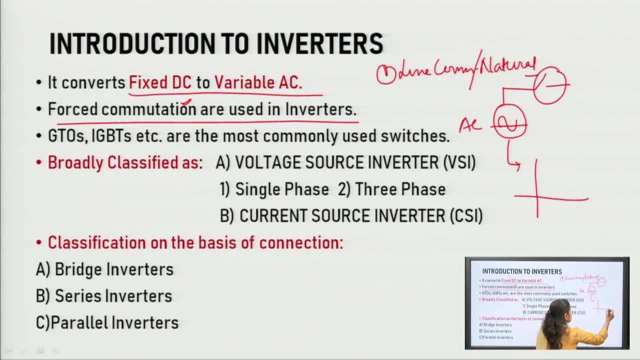 of AC supply. After positive half it is zero at this point and after this a negative reverse voltage is obtained here. This is the property of AC supply. Okay, This is AC sinusoidal waveform. So if on this switch from here, that is, from the input side, after some time a zero. 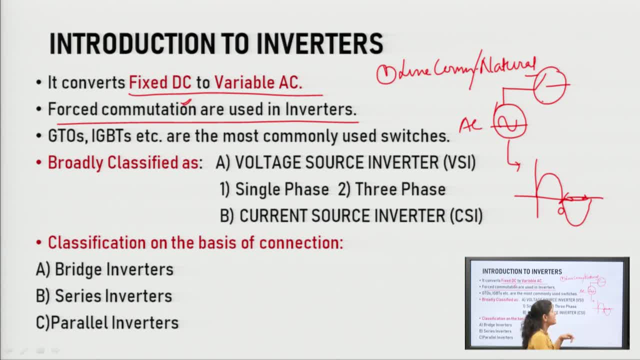 voltage comes and after that a negative reverse voltage is obtained, then this is basically the requirement to turn off any circuit, that the current flowing across it, the anode current flowing, its value becomes zero and then from here it gets a negative. 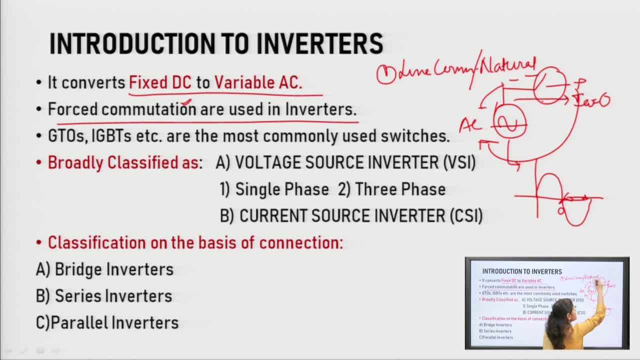 from here positive and this negative, a reverse bias voltage is obtained across the switch. This is the requirement to turn off any circuit, that the anode current flowing across it becomes zero, and after that a reverse bias voltage is obtained across the switch. 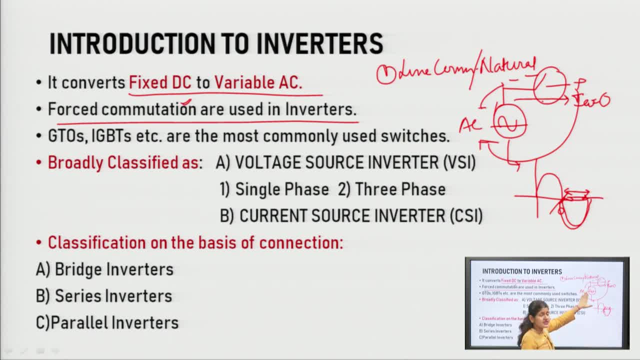 So this is the type of commutation in which the electrical supply which is the main supply, the AC sinusoidal supply, with the help of which we can switch off this circuit automatically. We do not have to put any separate commutation circuit to switch off this switch or to stop. 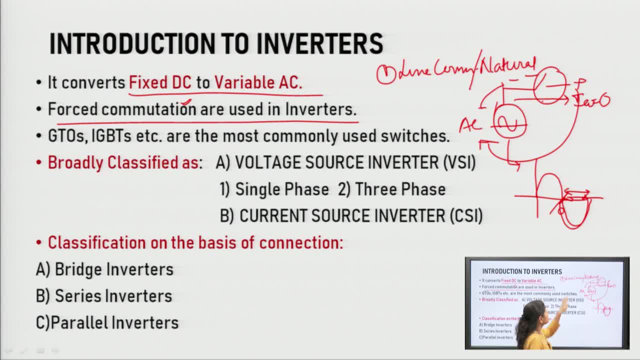 the conduction of this switch or this device. Okay, So this comes in line commutation. The next type of commutation is force commutation, which we generally use in inverters. Force commutation is unlike line commutation. Line commutation is generally being used where there is AC supply. 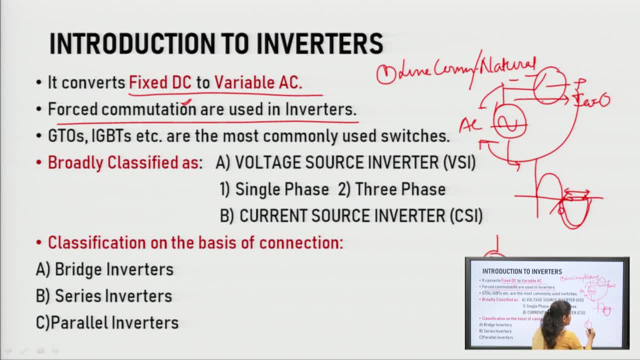 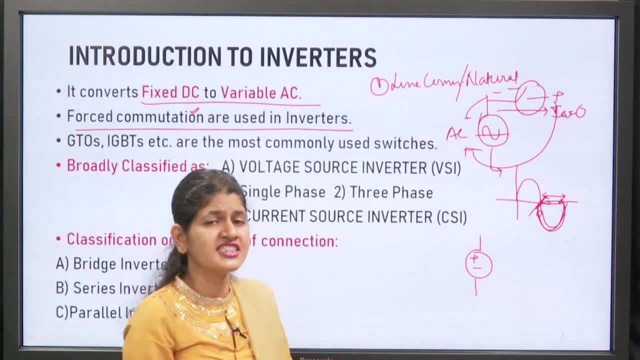 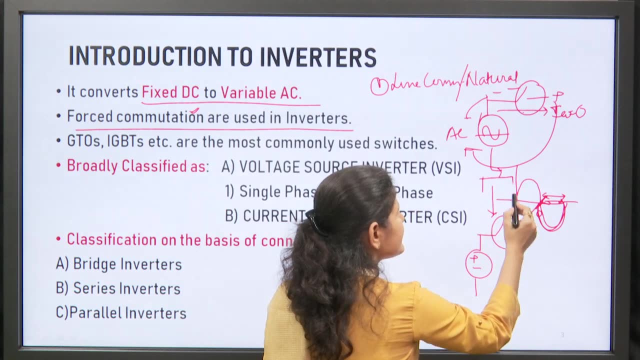 So wherever there is a DC input, wherever there is a DC input where there is no facility to go from zero crossover to negative, there, in the case of such inputs we do force commutation. So we have to put a separate commutation circuit to turn off this thyristor to turn. 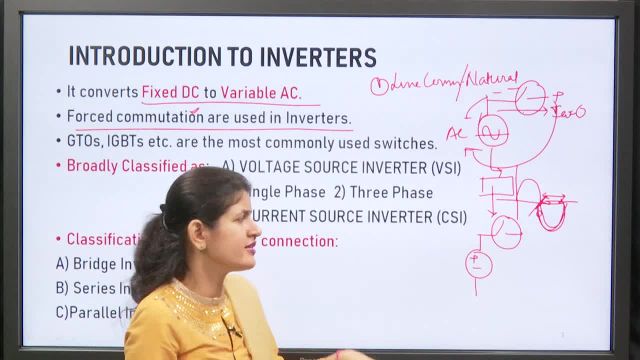 off this thyristor or whatever switch we people are using here. Okay, So this is force commutation which we use in inverters. One more small thing is that if we want to save the force commutation that we do not. 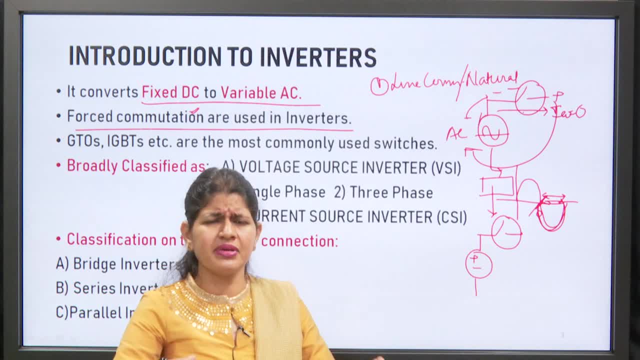 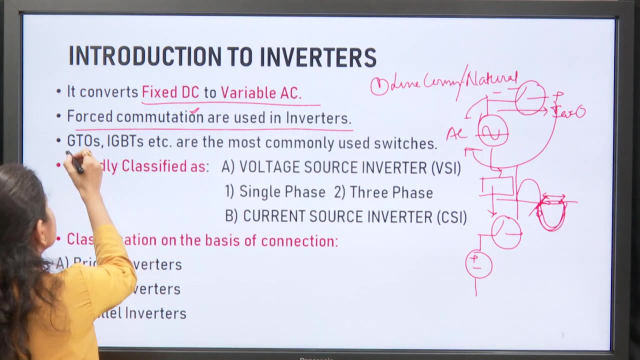 put a separate circuit in the force commutation because it also has its several disadvantages that the cost will increase and the circuit configuration will increase. Okay, The circuit configuration will be more complex because there is an additional circuit in it. So if we want to save these disadvantages, then we can use some of these types of switches. 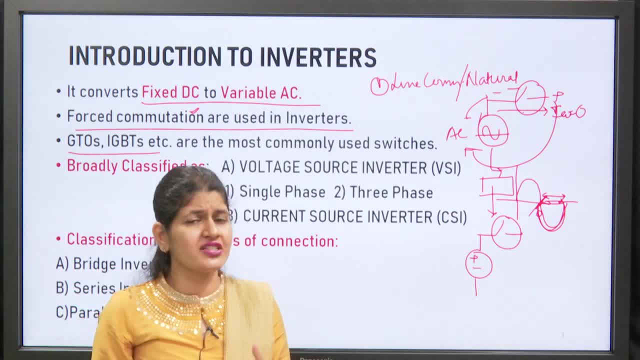 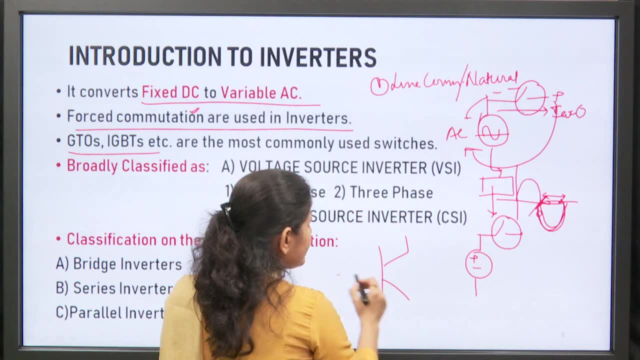 like GTOs, IGBTs. What kind of switches are these? These have automatically self-commutating properties. For example, we know GTO In GTO, the current pulses that we give from the base in this direction. right, that helps. 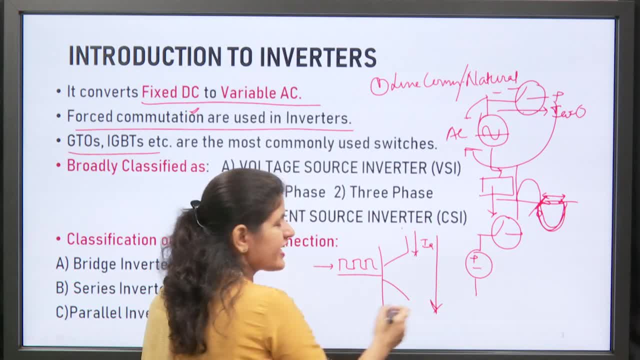 the IEA, the anode current, in this the cathode flow from the anode to here. Okay, In case that the anode current's flow, or that the conductions of the circuit is drawn in the direction of the ran current, the current running through the gate, or that we are giving 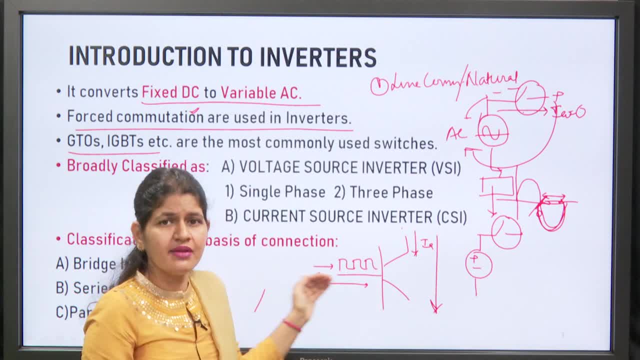 the current pulses helps it in its conduction. If we give reverse current or negative current, then what does it means? We are sweeping out the charges reduced in conduction from here. That is, we are pulling out. If we will pull out, then this help that we were getting will that help to conduct will. 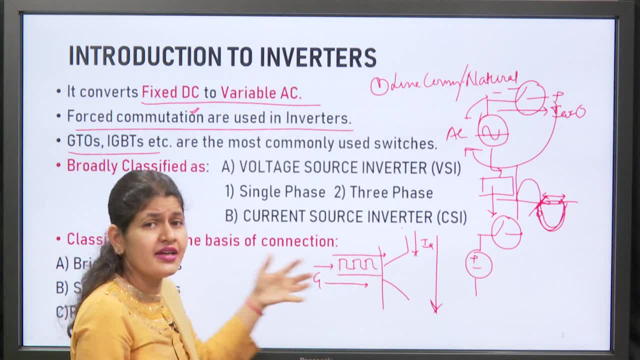 stop right. This will stop where the current in the diodes is kept and consequently the needs of the diodes are until the i3,. so all that. So the power is equal in foot, in относguy right. 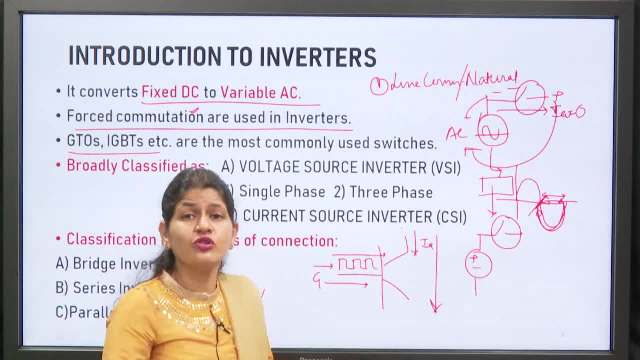 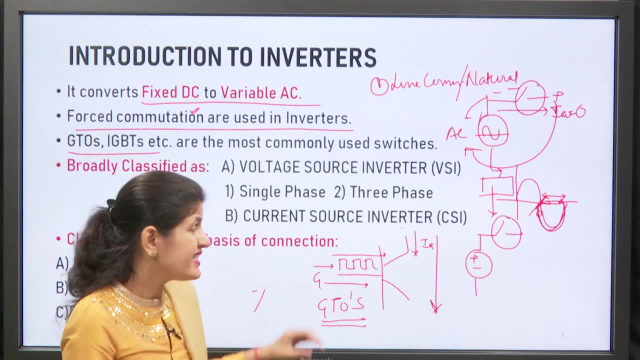 conduction karne mein, wo madad rukh jayegi to ye conduction bandh ho sakta hai, the GTOs or IGBTs kuch aise self-commutating devices hain, jinke base ko transistors mein gate. 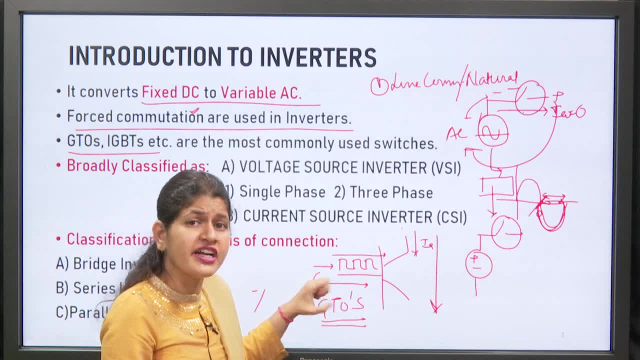 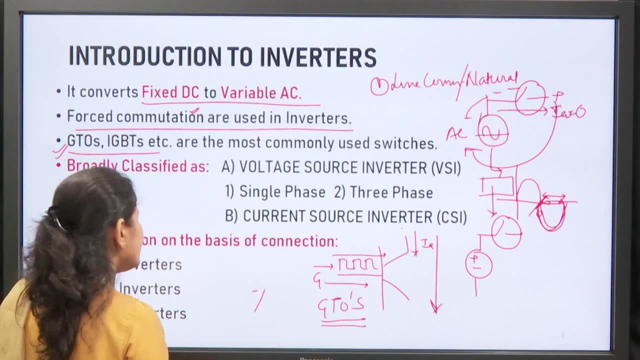 ki jaga base hota hai. to jinke base ko, ya gate ko control karke hum is circuit ko turn off kar sakte hain. to is tarike, ke switches inverters mein use karte hain. ab aate hain. 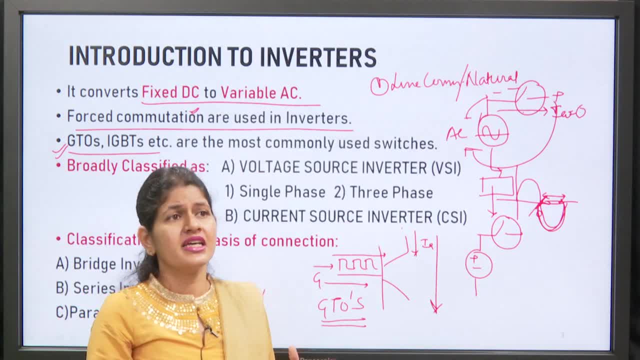 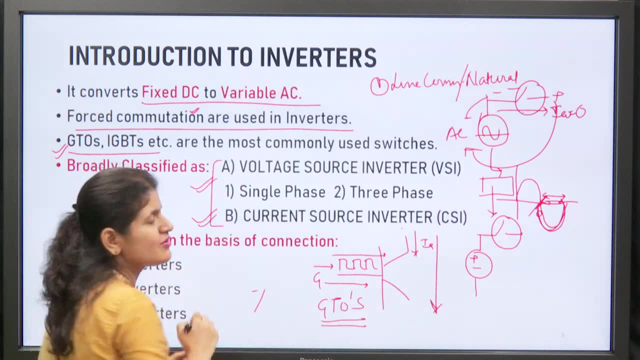 further classification pe to jaisa ki humne baat ki thi abhi, ki alag alag tarike se classify karte hain, to sabse pehle broadly classify hota hai: voltage source inverter or current source inverter. mein iski next usme hum log baat karenge, ki ye dono alag alag hain kya. 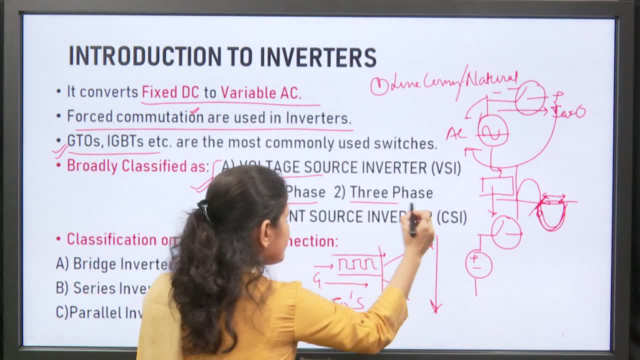 to voltage source, inverter bhi further, single phase bhi hota hai, three phase bhi hota hai. theek hai to ye ho gaya do tarike ka classification jo hum broadly kar rahe hain on the basis. 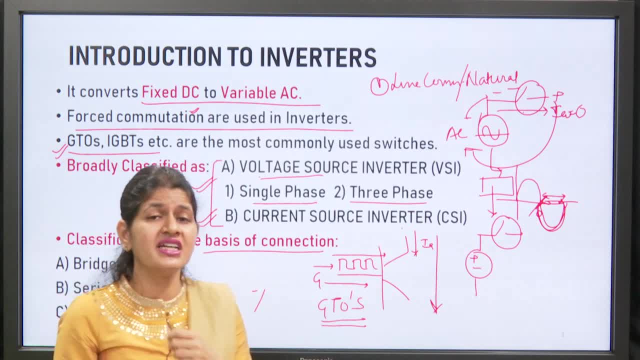 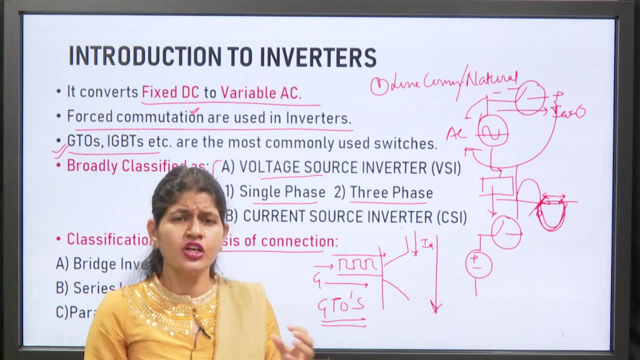 of connection on the basis of connection of power semiconductor device. used power semiconductor devices thyristor family ke har element ko hum power semiconductor device kah rahe hain to unka connection, kaise laga hai usse configuration ke basis pe further? 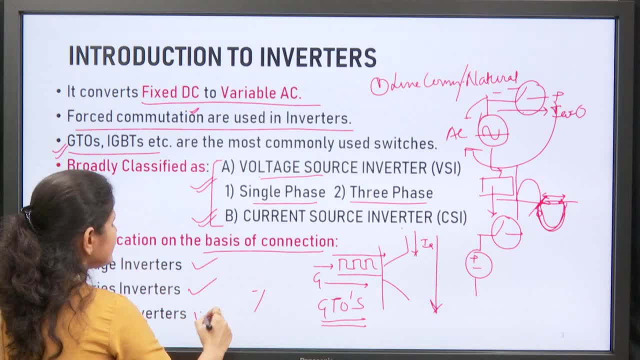 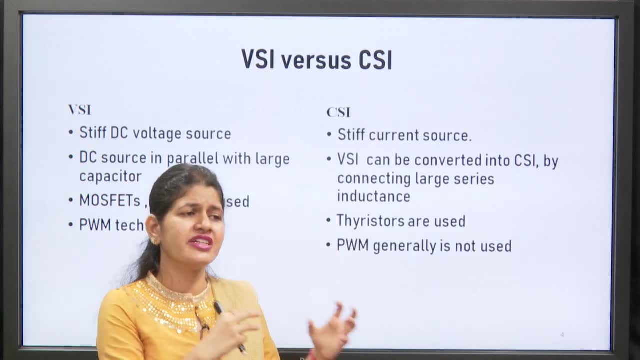 teen classification hum karte hain: bridge inverter, series inverter or parallel inverter, theek hai. Next dekhte hai vsi versus csi, dono hi dono, voltage source inverter or current source inverter. mein difference kya hai to voltage source inverter? kya hai jaisa ki sunge samajh. 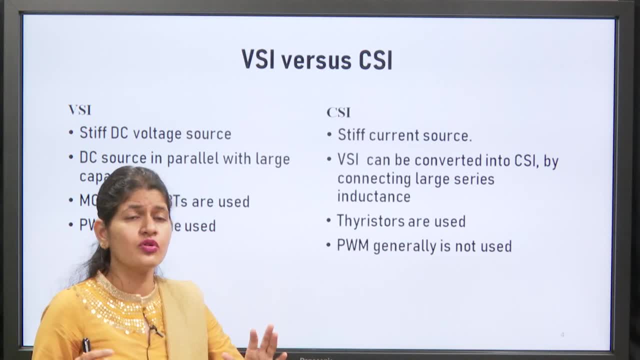 mai aara hai ki voltage source inverter is jisme source voltage ho aur current source inverter hi is jisme source current ho. Something we can understand is that which is specific difference for voltage source inverter's. voltage source inverter is source current, current source. is it real voltage source 취 Pourquoi so? 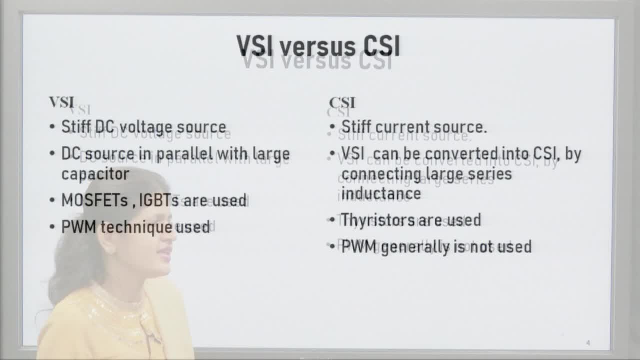 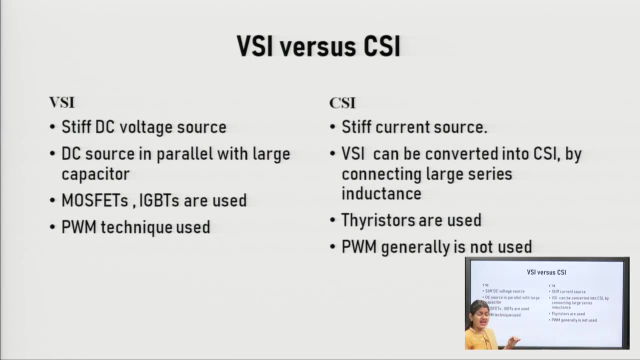 So we know that there is no such thing as a current source in general. So a current source is made with the help of a voltage source Before that in a voltage source inverter, if we want a constant voltage or stiff voltage in the input side. 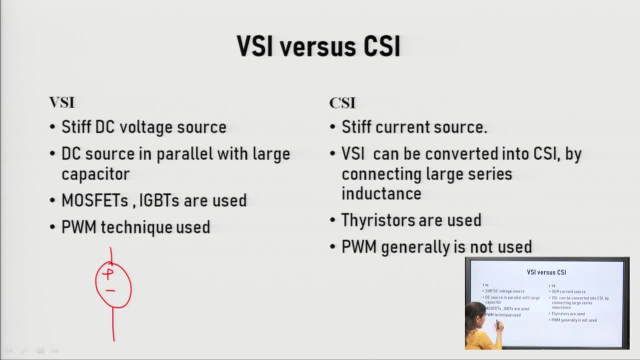 then what we can do is if a high value capacitor is installed in parallel of a voltage source which stores high positive here and high negative charge here, then it helps in maintaining or upholding its constant voltage. So in a voltage source inverter, if a high value capacitor is installed in parallel of any voltage source, 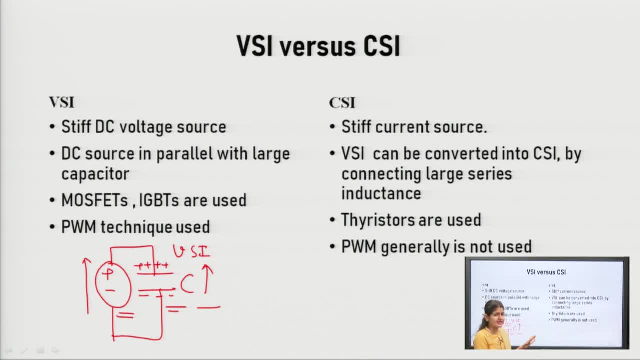 then we can make a voltage source like this. Now, as we discussed that CSI is made with the help of voltage source, then if a high value inductance is installed in the series of voltage source, then what is the property of inductance? 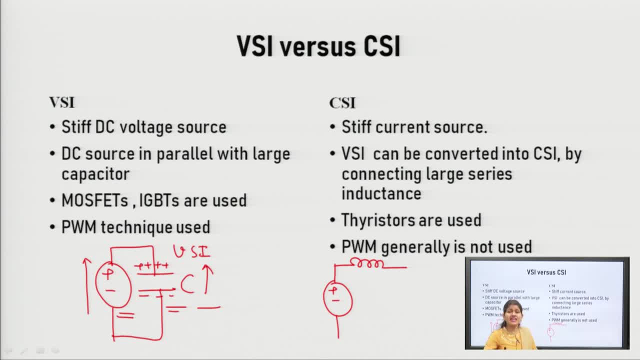 Inductance itself does not allow. the rate of change or instantaneous change That is, the current coming out from here, cannot be very instantaneously. the ratio of DI by DT cannot be very high. sorry, the rate of DI by DT cannot be very high. 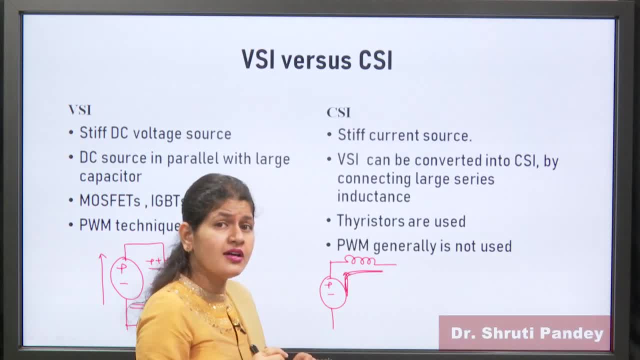 So a current will flow continuously from here. Second, along with the magnitude, the reverse of current also does not allow the inductor. That is, if the current is flowing in this direction, it will flow in this direction only. Okay. 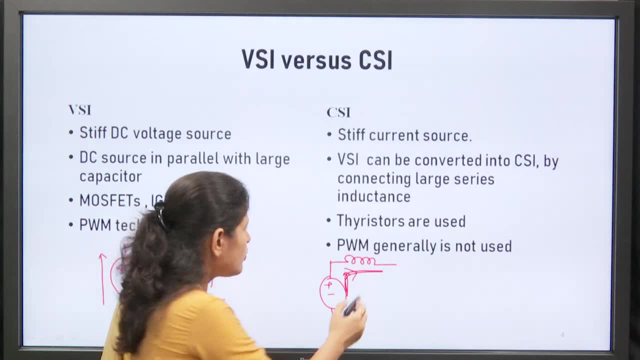 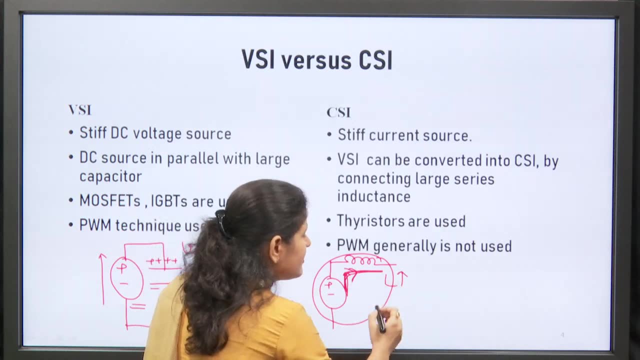 So it does not allow the reverse of current instantaneously. Okay, So, along with this, because a constant current can be obtained here because of the high value of this inductor, then CSI is made along with this Current Source Inverter. 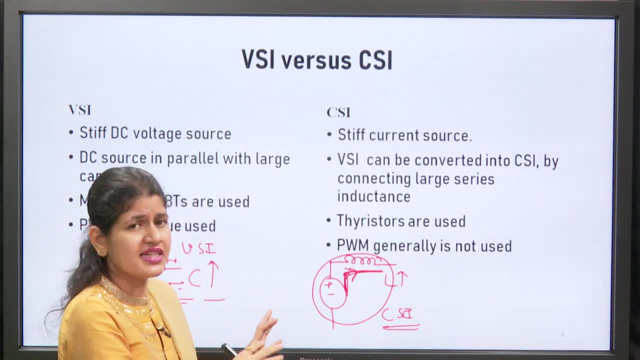 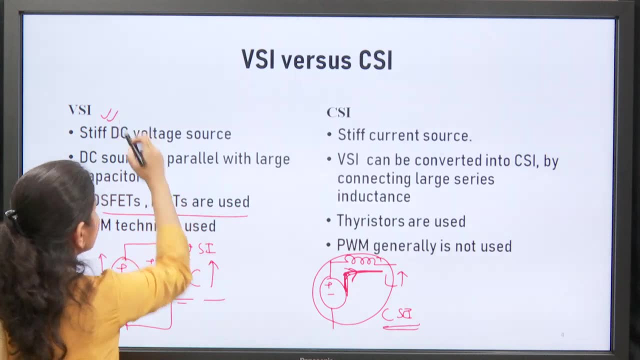 Okay, So this is a big difference in CSI and VSI in terms of configuration or appearance. Next, we use MOSFET and IGBTs in VSI and we use thyristors in CSI, In voltage source inverter. 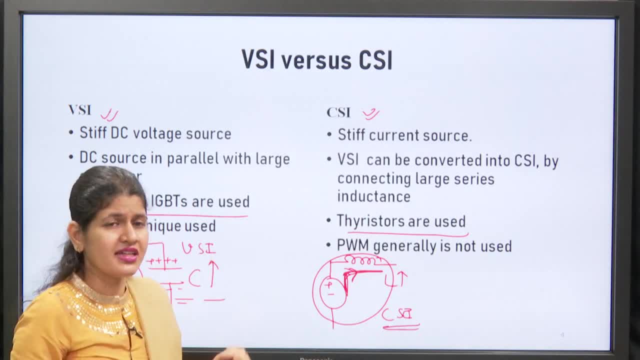 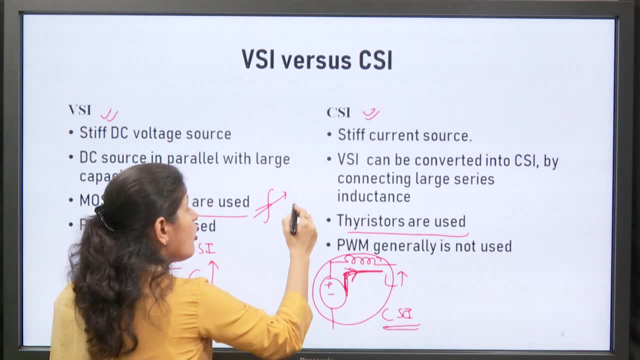 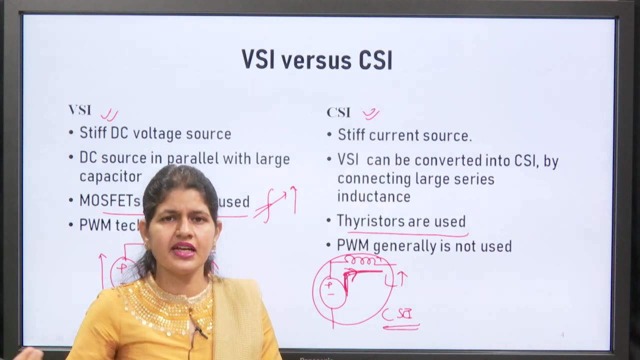 these two types of switches are used. And what do I mean by these types of switches? High switching frequency devices whose switching frequency is very high. High means- and you must have already known that- MOSFETs and IGBTs, these types of power semiconductor devices. 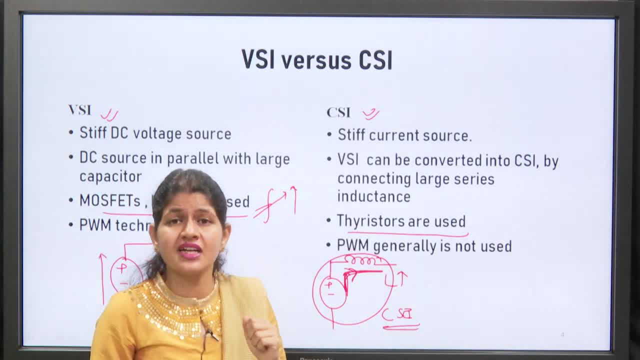 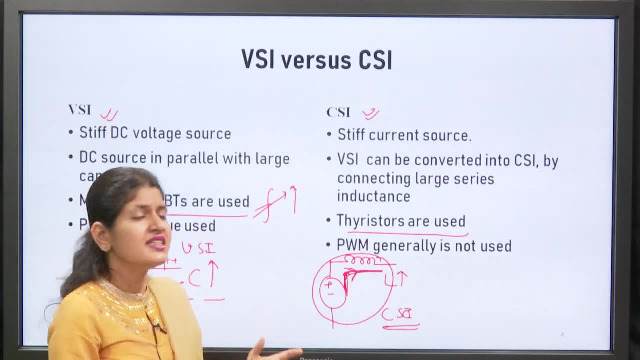 their switching frequency is very high compared to thyristors. What does higher switching frequency mean? On-off control Switch's on-off can be done much faster Or can be done at much higher speed in this higher switching frequency device than thyristors. 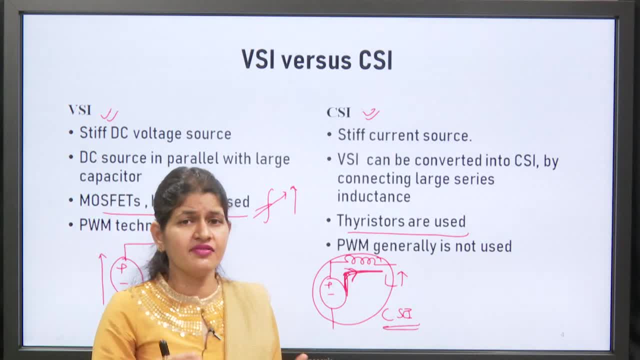 Where this higher switching frequency comes, there comes one more thing, which we call harmonics. The higher the switching frequency means the faster the switch will switch on-off, on-off, the more harmonics will be there. Okay, So because of this, 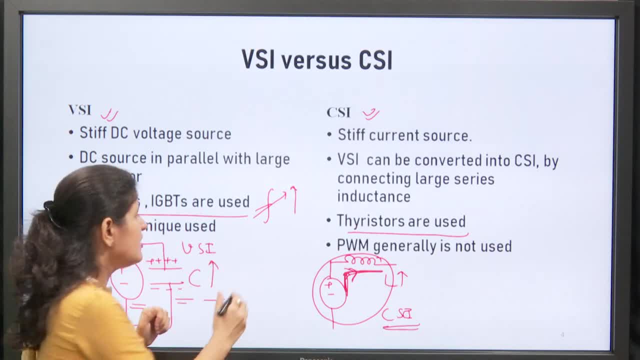 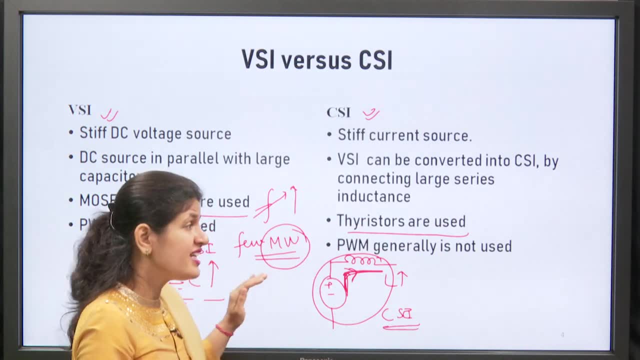 a limitation comes here: that the VSI's can be used only up to few megawatt range. That is, few kilowatt to few megawatt range only can be used. That means their power handling capacity is less, Whereas 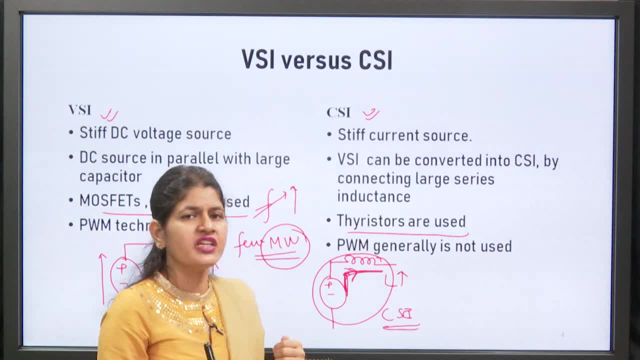 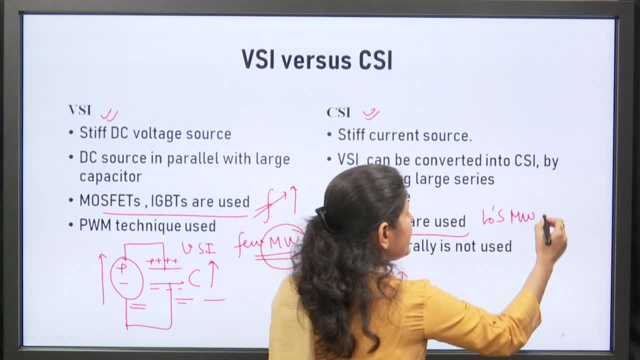 in thyristors. because of slow switching or low switching frequency, the harmonics will also be less So. because of this, tens of megawatt- tens of megawatt means in case of higher power handling capacity, we use thyristors. 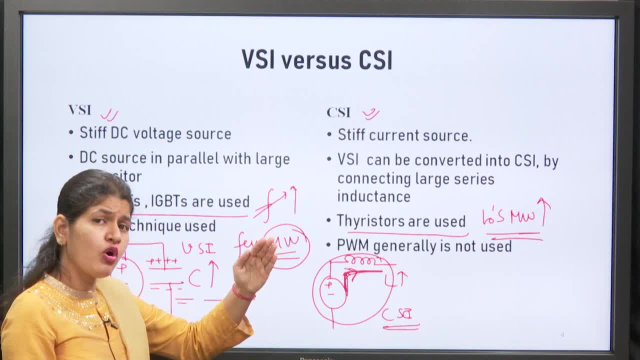 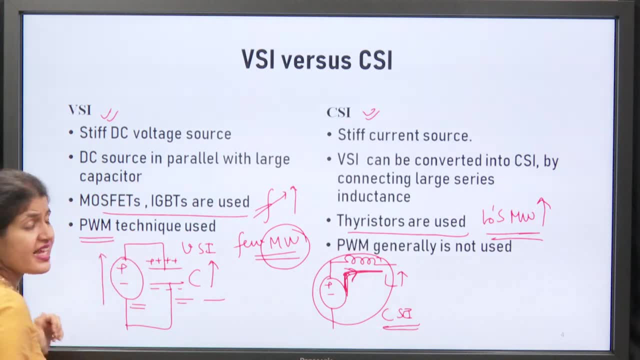 Apart from this, where we talked about that, we can switch on-off fast there, in both the control of inverters. here we use a technique- it is called PWM technique- Pulse Width Modulation- which we will read in detail further. 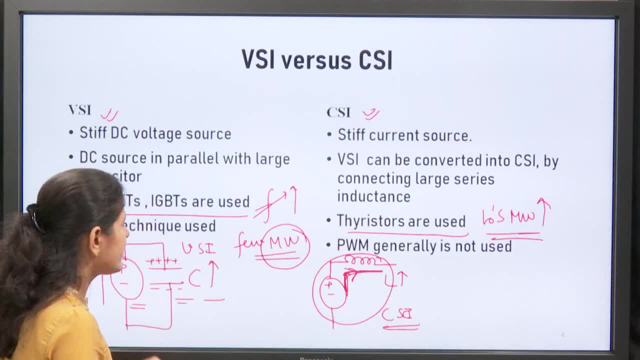 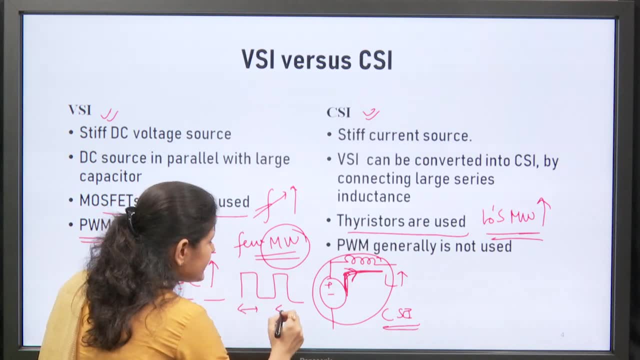 because it is a very important topic. Okay, So Pulse Width Modulation now. basically, by listening, you understand how to modulate the width of the pulse. This is the pulse, this is its width. So, by modulating the width of the pulse, 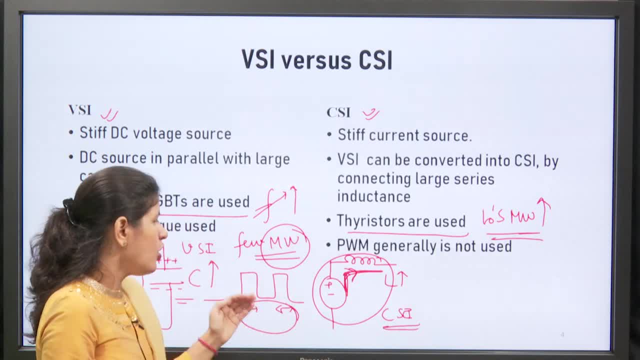 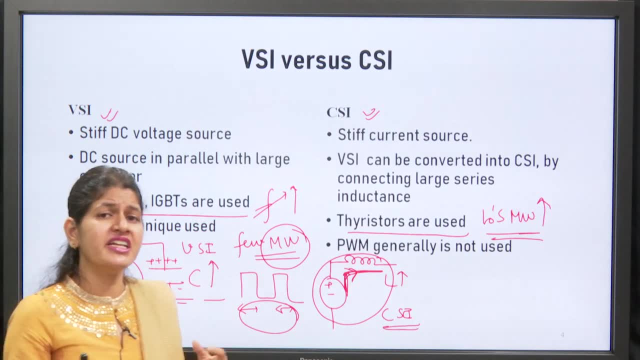 we put a control mechanism in it And the width of the pulse. why are we using the Pulse Width Modulation technique in VSI? Because the higher switching frequency devices, these are the devices which are on. then conduction happens. 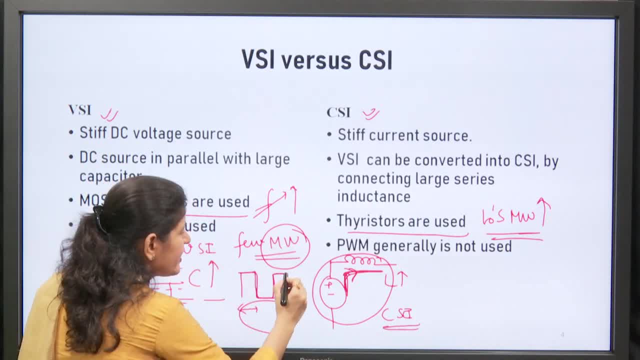 means we get this type of output. if it is off, then zero, if it is on, then like this: if it is off, then zero, Whereas this does not happen in thyristors. If you switched off immediately. 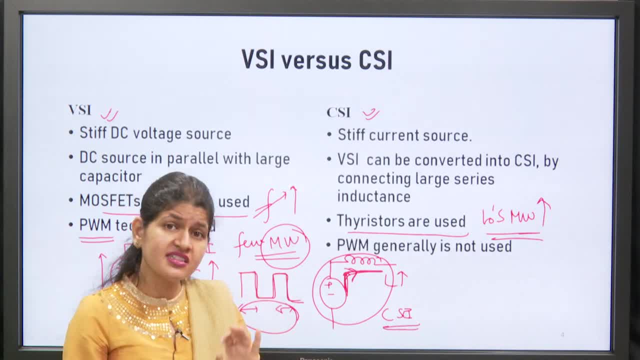 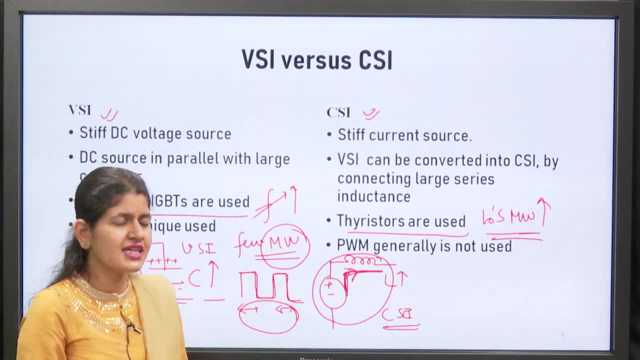 switched on immediately, then it is not necessary that as soon as you switched off, the thyristor stops or the conduction stops across the thyristor. it takes some more time. That is why we call them higher switching frequency devices. 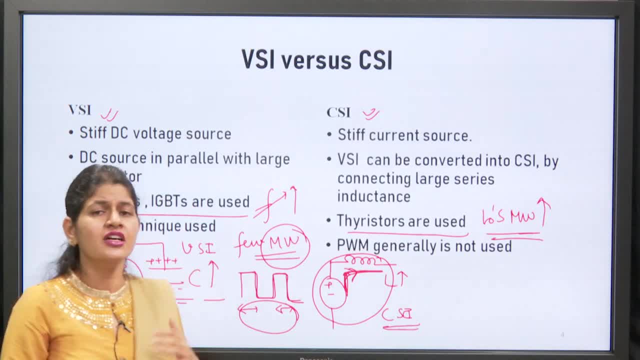 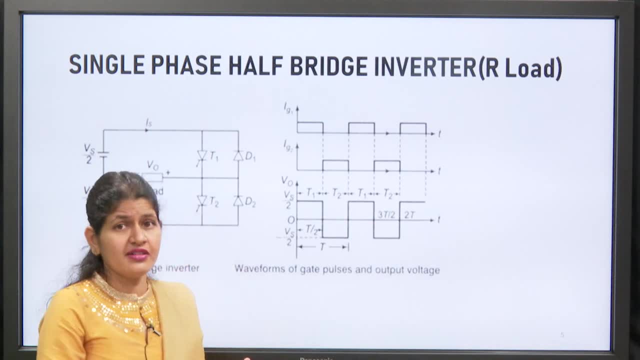 That is why these higher switching frequency devices are used in VSI And that is why we can easily apply PWM technique in VSI. Okay, Next, let us come further, the second classification, which we will move on to further in the VSI classification. 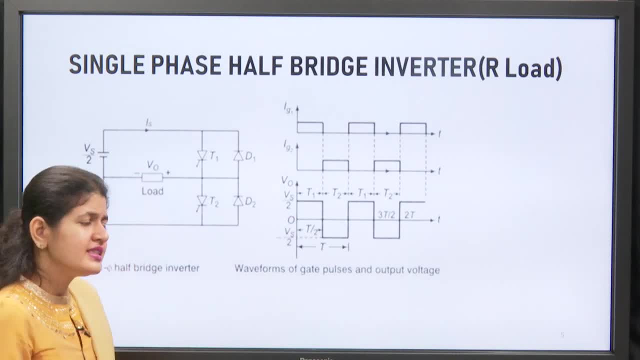 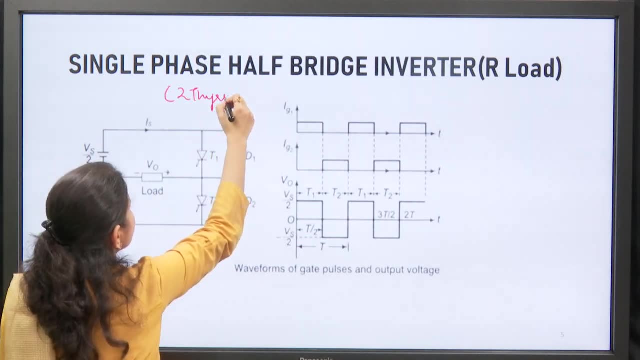 that is Single Phase, Half Bridge Inverter. Okay, So in Half Bridge Inverter. first, how many thyristors are we using? We are using two thyristors in it. Okay, Two thyristors or any switch. 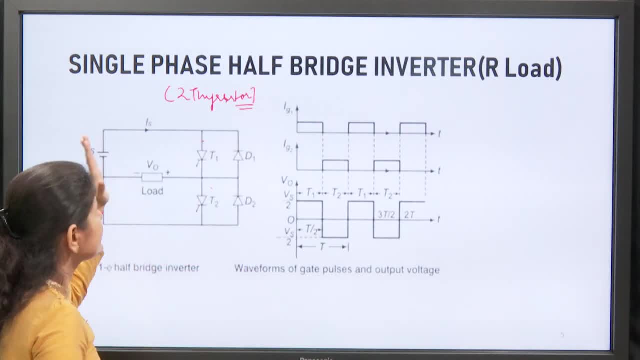 we are using two, one and two In the same way. the single phase full bridge will come. when we will read next, then we will see that we are using four thyristors in it. So anyway, first of all, 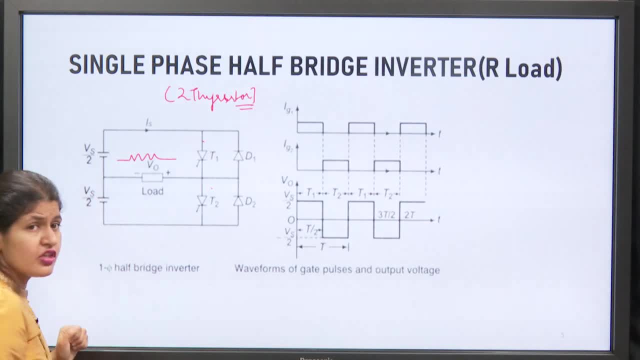 let us see with R load. If here R load is applied, then this inverter, Single Phase, Half Bridge Inverter, how will it respond? First, when upper half of VSI2 comes, upper half, lower half is given. 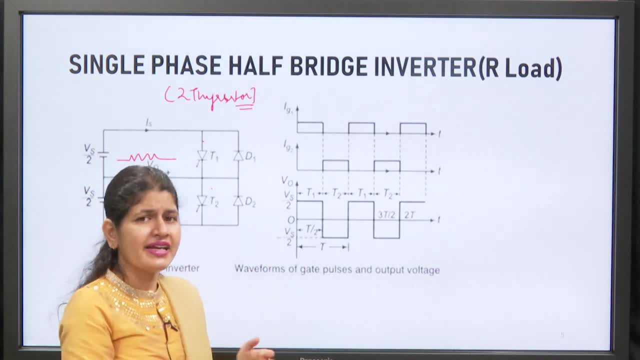 then here one more thing comes, that how this type of supply is applied in it. This type of supply means above plus VSI2, and below plus VSI2,. this type of system, we call it three wire system. 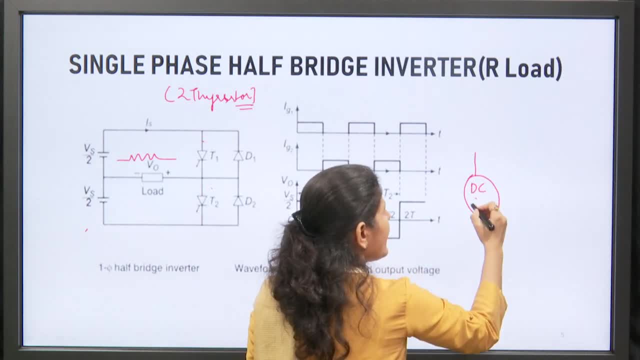 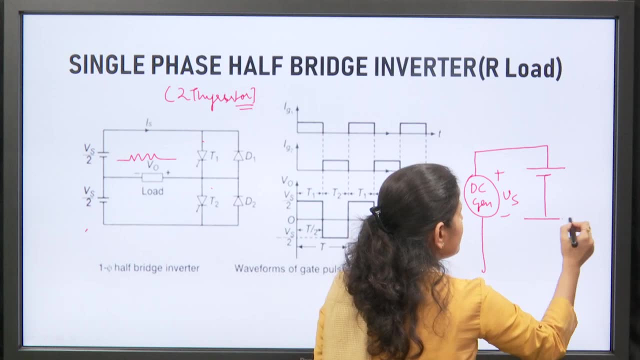 Okay, Three wire DC system. In this what happens is, whatever is the DC generator here, it generates plus minus VSI, and this we further here VSI2, and here VSI2, means balanced. this is balanced VSI2,. 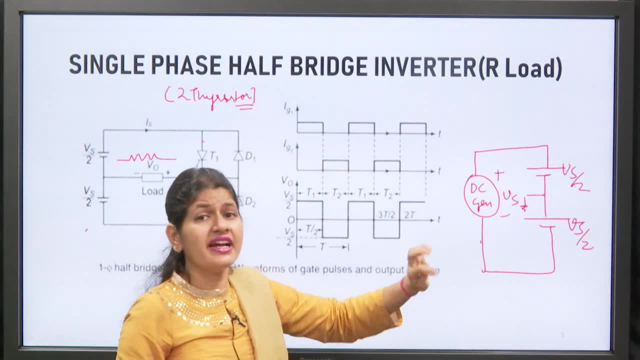 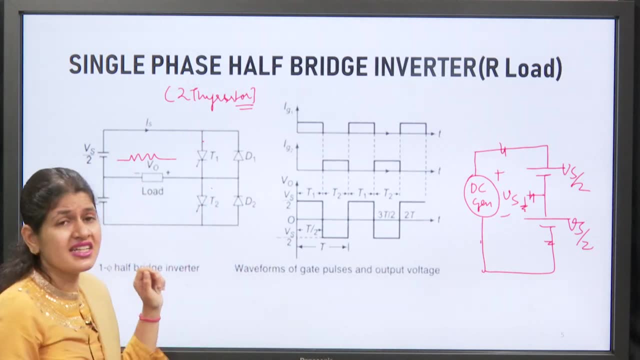 with the help of this neutral. in this way, this we call three wire DC system. Okay, So, in this, one is this wire, one is this wire and one is this wire. Okay, So we use three wire DC system. 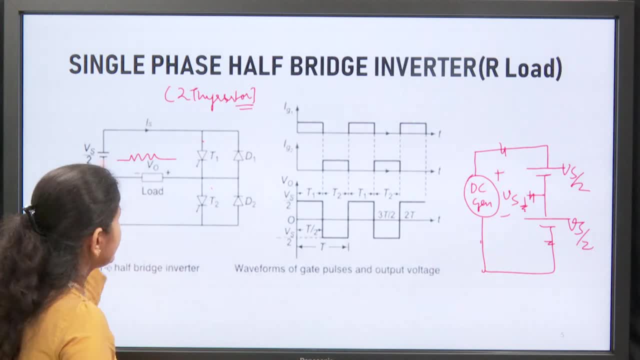 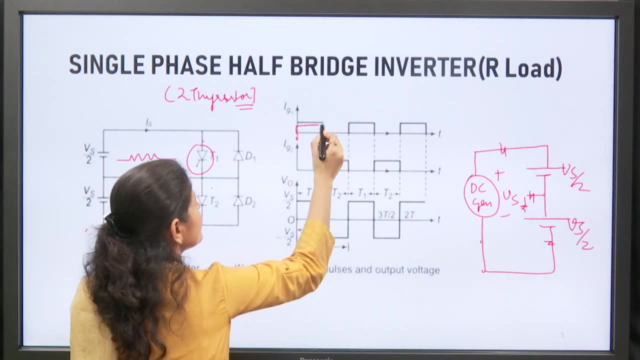 single phase in half bridge inverter. Okay, So see in positive half cycle, what will happen When we triggered the thyristor of T1, where, At zero instant- see- we triggered the thyristor of T1.. 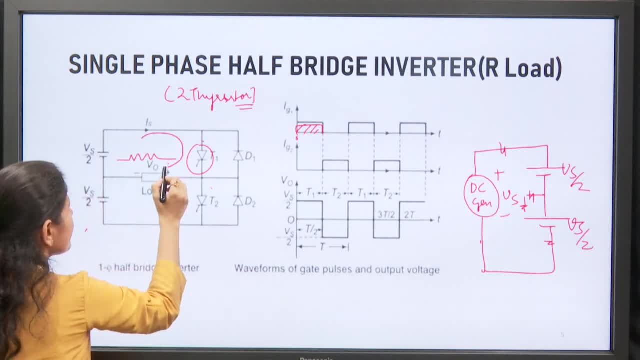 Okay, So how is the current flowing? The current is flowing in this way. this IS current. If the IS current is flowing like this, means the current is always flowing from positive and goes till negative. Okay, So the current is flowing like this. 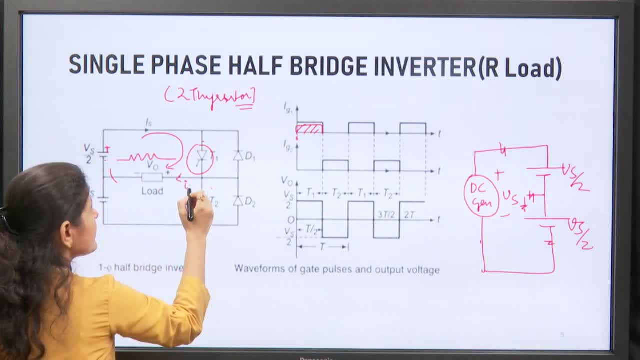 so this is the direction of I0, and the I0 is flowing from here to here. so here is plus and here is minus. So whatever load is there on its left terminal plus, and on the right, 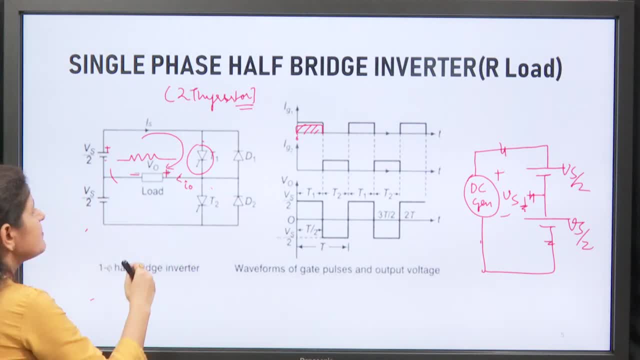 minus polarity is being formed. Okay, So in this way, how much V output we are getting When T1 is on? so how much V output we are getting? We are getting V output plus Vs by 2.. Okay, 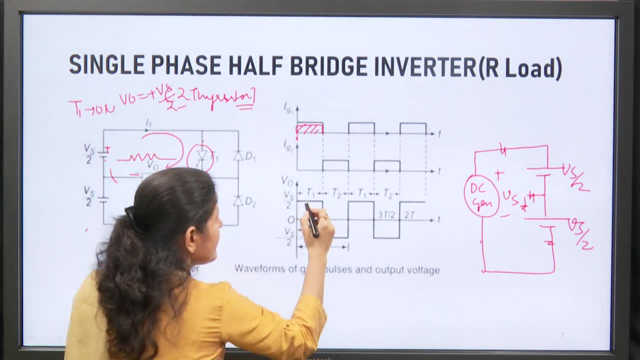 This is also visible here: plus Vs by 2, right, This is plus Vs by 2, this is the magnitude we are getting Now when we at this point at T by 2 time. if this whole time is T. 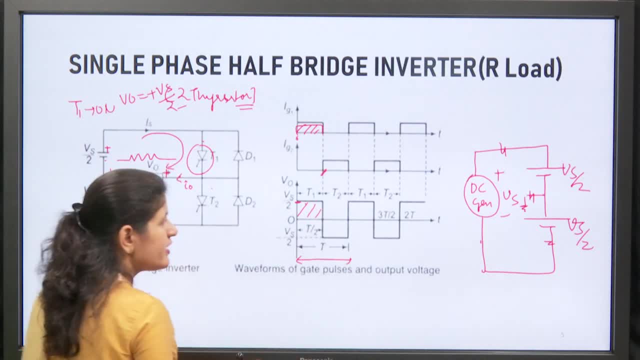 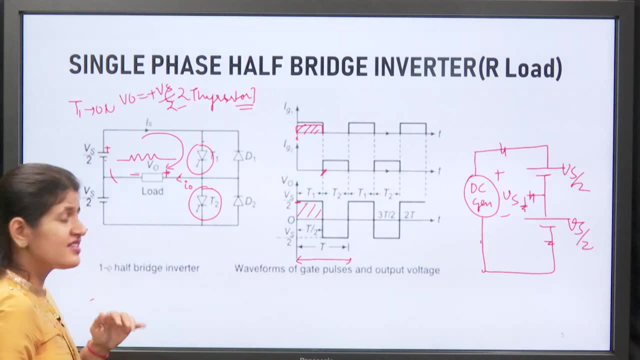 then this instant is T by 2, now T by 2, this instant, at this instant, we are turning on another thyristor, Which one? T2 thyristor? When we turn on T2 thyristor, 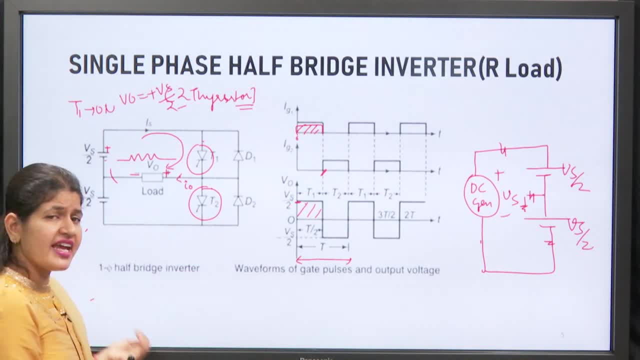 then what will happen? As always, current will go from positive to negative. That means from this positive across this load. here a resistive load is applied. current is flowing across that load, like this, right From positive. 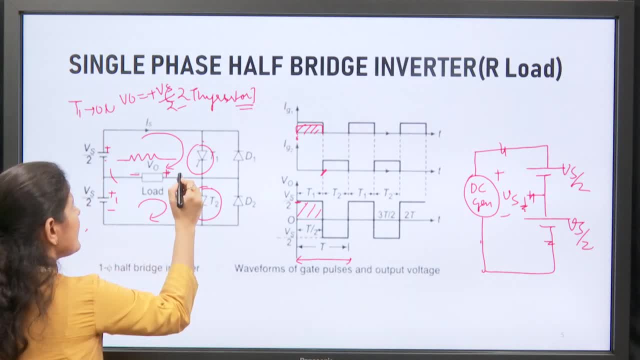 it went to anode and back to negative. If we assume this reference as the direction right, Assume this reference as the direction of current and voltage polarity. if we assume this reference as the direction, then T1, which is conducting. 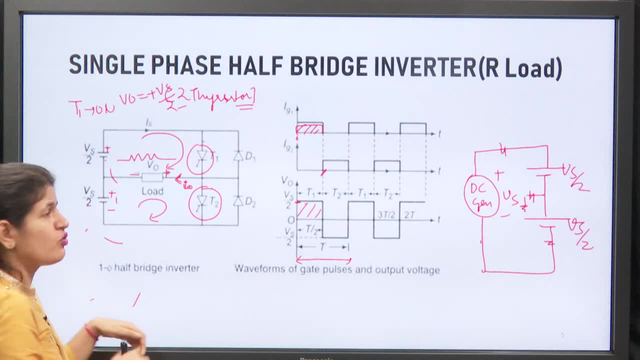 if that reference is there, then now see, current is flowing in opposite direction. Right Current is flowing in opposite direction. Earlier current was coming like this. now current is coming like this, So current is also flowing in opposite direction. 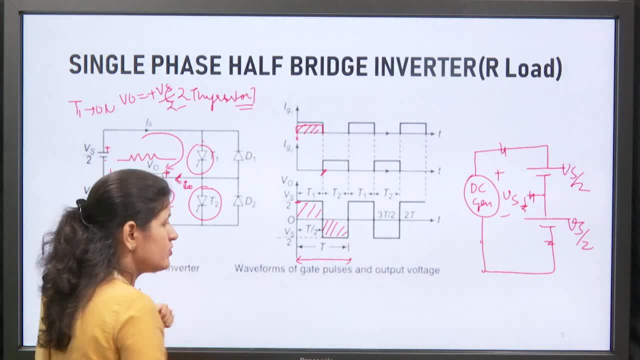 and voltage polarity is also coming opposite. Because of this, in negative half we get minus Vs by 2.. Minus Vs by 2, and below this its current waveform will also be formed. Current waveform will be just like this. 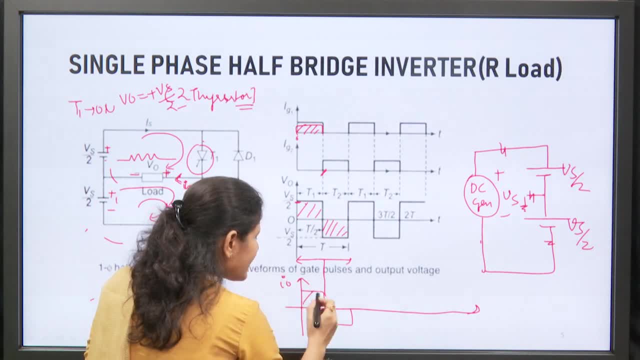 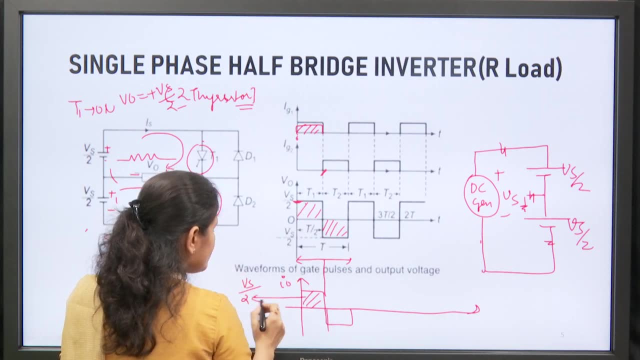 just like voltage waveform: I0 waveform. Just its magnitude. how much will it be If this voltage was plus Vs by 2, then what will be the magnitude of current Vs by 2 upon R? In the same way, 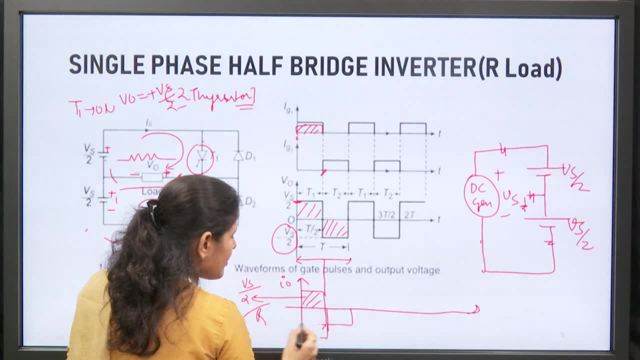 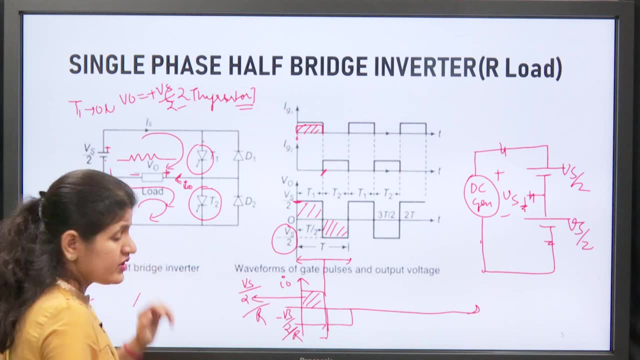 if negative magnitude was minus Vs by 2, then how much will this magnitude be Minus Vs by 2 upon R, V by R? This is the I0 current Right. So this is the single phase half inverter. 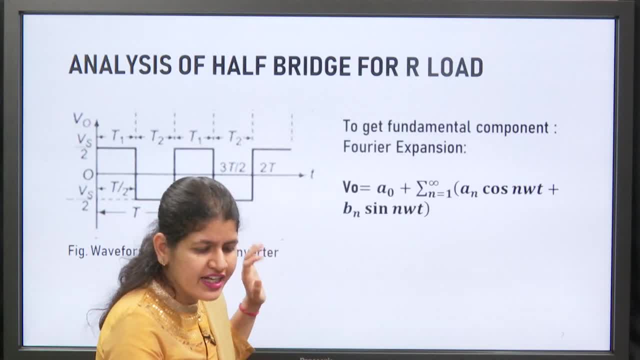 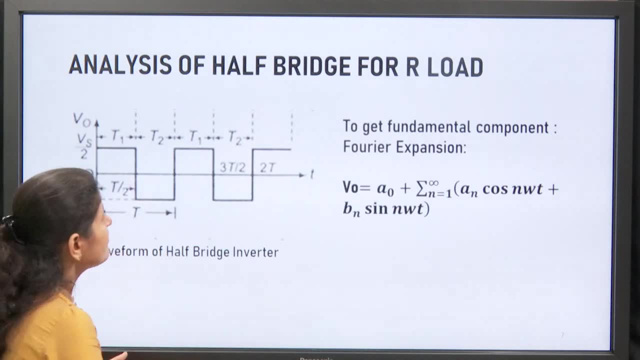 One more small thing here. this is the description of that. only One more small thing which is here, that is, to do its analysis, To do its analysis in analysis. basically, we will do analysis through Fourier expansion. We will look at this further. 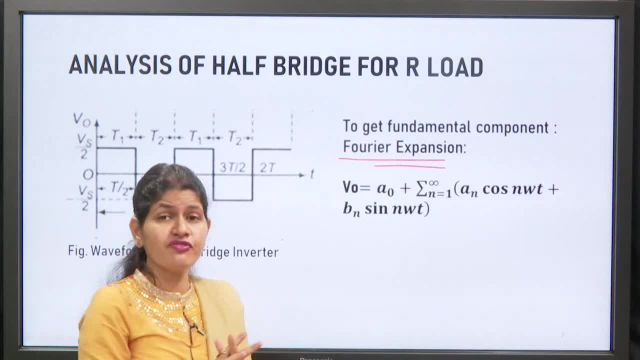 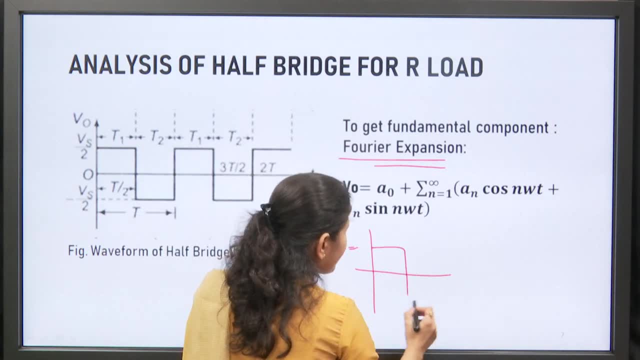 in full wave But in analysis. basically, we will know that. why do we do Fourier analysis? We do Fourier analysis because if we are getting any square wave waveform at the output, at the output, if we are getting such waveform at the output, 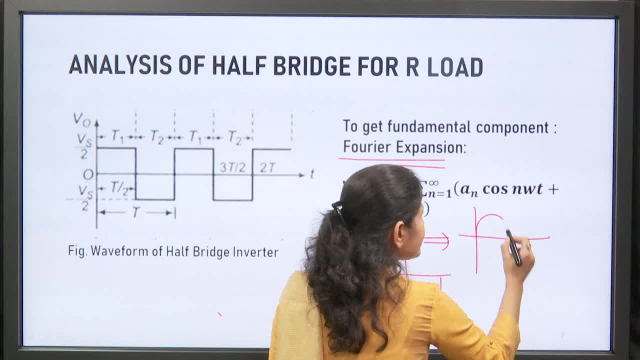 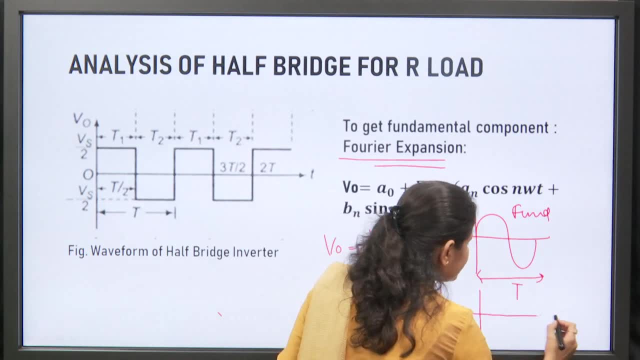 then in which elements it can break further. One will be its fundamental component. Right, If this frequency is T, then this is its fundamental component. And in the same way, in the same time, T in the same time. 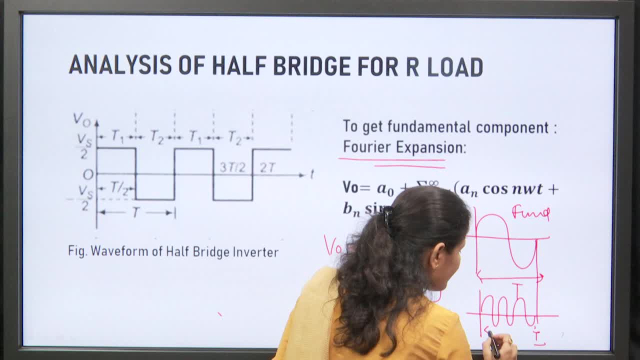 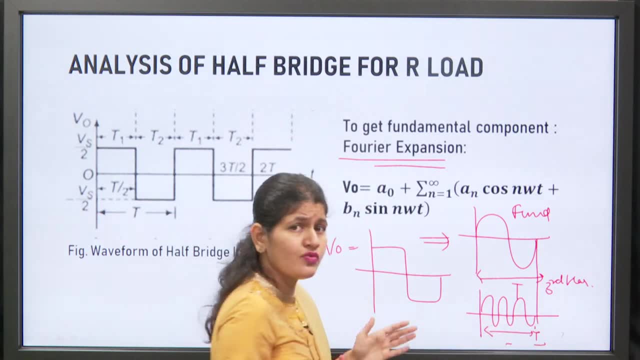 T. if one, two and three, three frequencies come, then this is its third harmonic component. Right In the same way, in the same time, if five cycles come, then it becomes the fifth harmonic component. So, 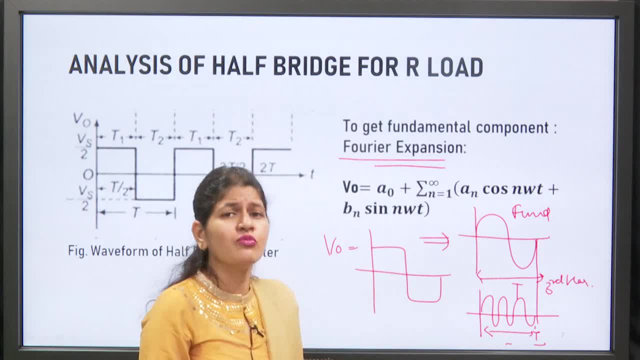 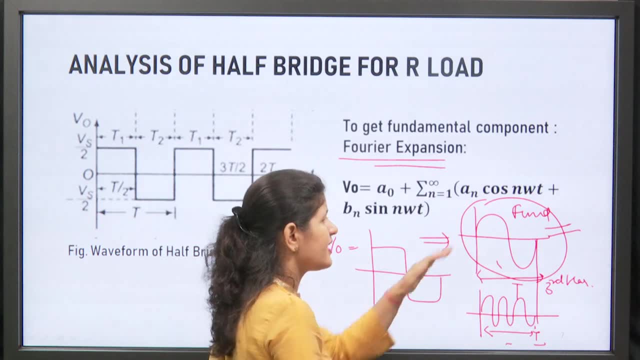 in one square wave, in one fundamental or sinusoidal waveform, there are several other harmonics also Right. So this fundamental waveform, which is desired because we want it at the output of AC, Apart from this fundamental waveform, 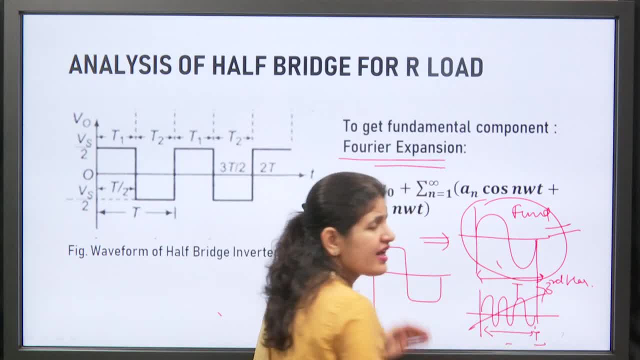 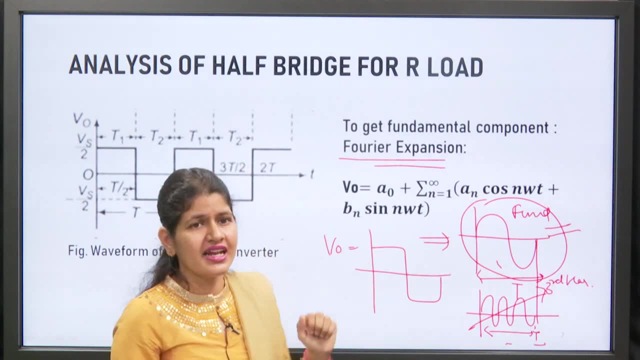 all these elements which we are getting, harmonics to separate them from the fundamental or to remove this separate element. we do Fourier analysis Right. So in the next further slides we will see here, we will see: 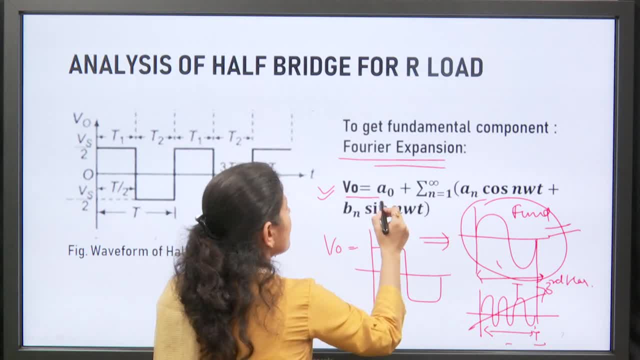 what is the expansion of V naught? V naught is A naught, which is the DC component. Apart from this, AN cos, omega cos, n omega t, which is the cos component, and sin omega t. So what do we get out of this? 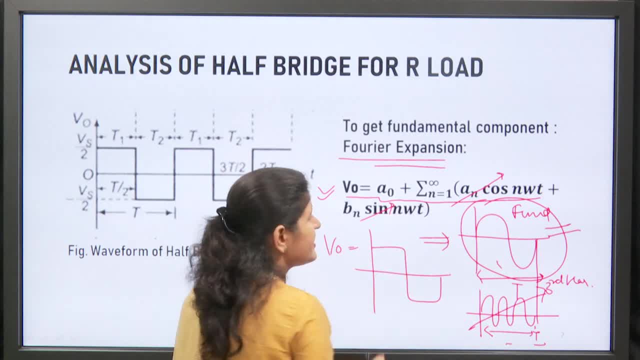 So we get, we get, we get what is required out of this. A naught is the DC component, which we don't want, Cos component, which we don't want, Which one we want, Sin component. So 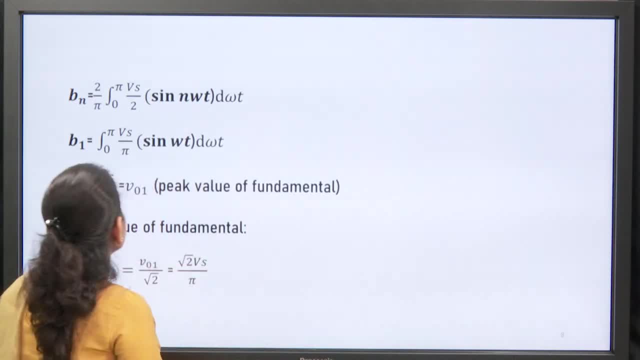 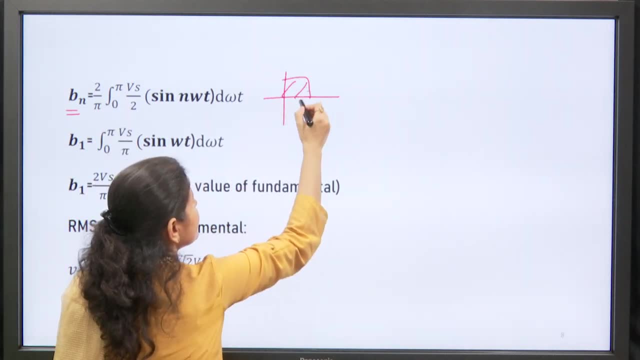 we will do its analysis Right. So you see, we have done the analysis of the Bn component 2 by pi, 0 to pi, because till the time of 0 to pi we are getting Vs by 2,. 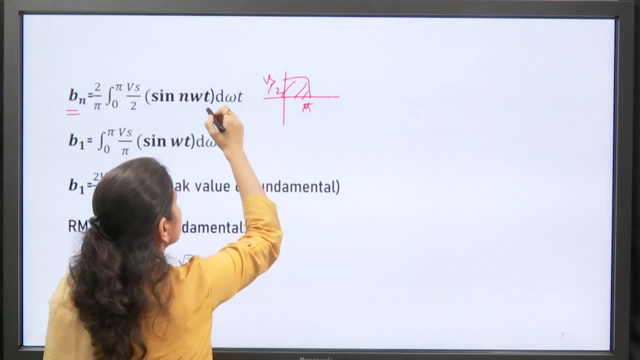 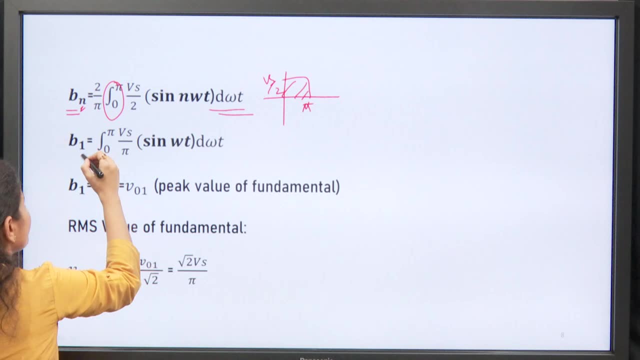 till the time of pi. we are getting Vs by 2,, so Vs by 2, 0 to pi In this. if we want the fundamental or first component, then we will keep the value of n as 1.. 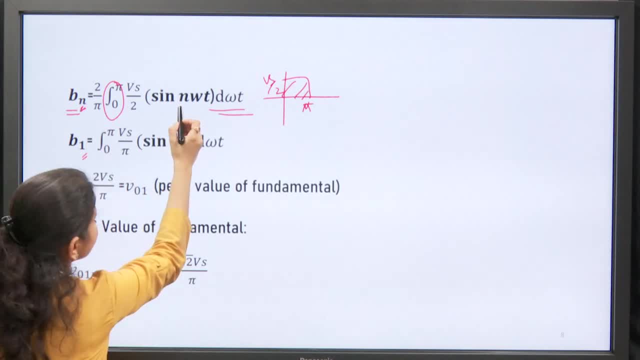 Right, We kept the value of n as 1.. So wherever the n component was coming, we kept 1 there. here also 1.. So this value of B1 came Right After B1, the value of B1,. 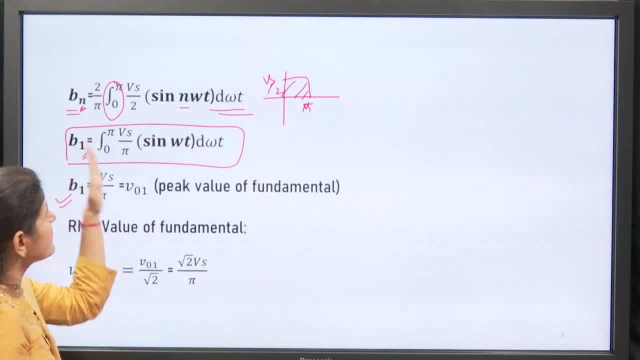 this sinusoidal. integrate it from 0 to pi. integrate this term. So what is coming? 2Vs by pi, which is V01.. Right, We have shown B1, V01.. This component, which is sinusoidal, 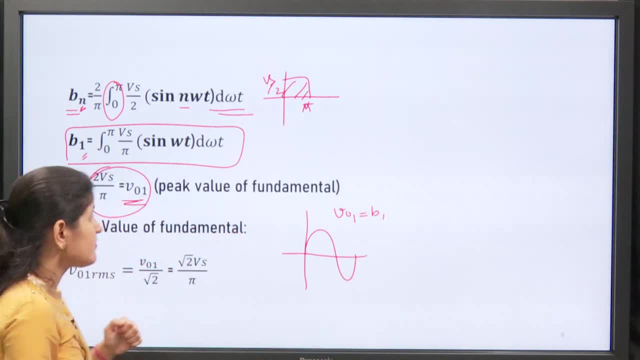 we are calling this as V01, or B1 component And this is we call this peak value of fundamental component. So fundamental component: V01's value. this has come Right. I have told you. this is the fundamental component. 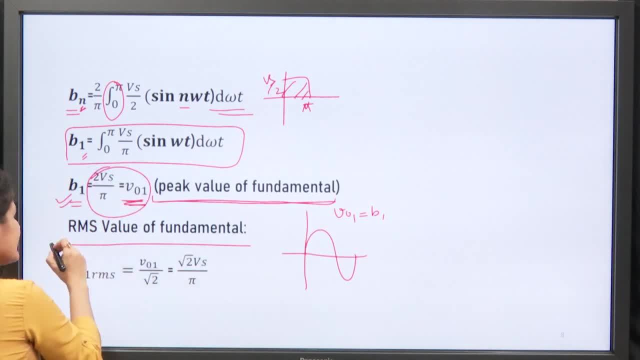 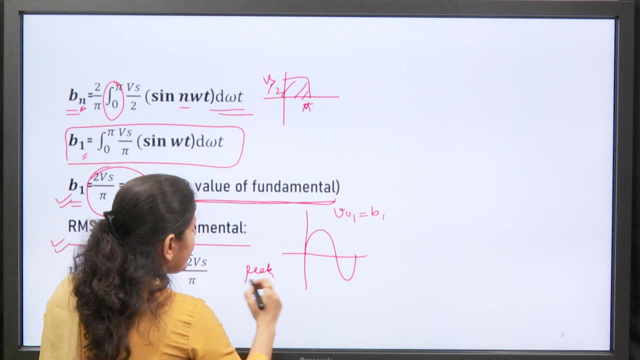 which we wanted. So this is peak value of fundamental. Now, if we want to get its RMS value, then what do we do? We know that peak value upon under root 2, right, Peak value upon under root 2,. 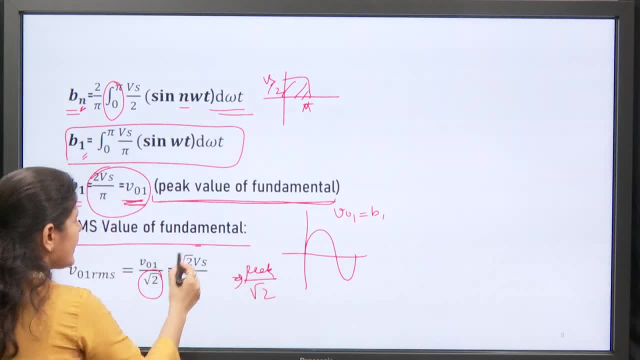 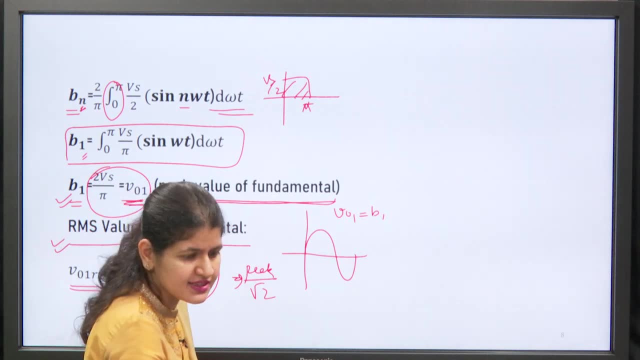 is RMS value Right? So upon under root 2, we got this RMS value. So what has come? RMS value of fundamental component under root 2, Vs by S. Now see we are doing analysis on AC side. 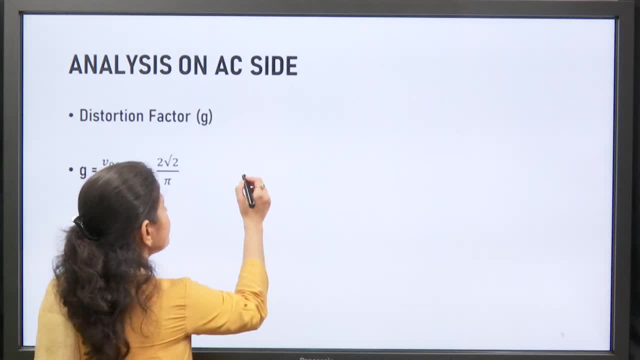 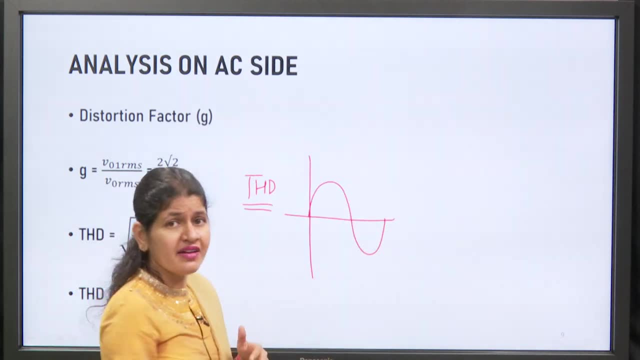 On AC side. how do we do analysis On AC side? we basically see that how much is the THD of output waveform, That means the one AC waveform which is available on output THD is total harmonic distortion. 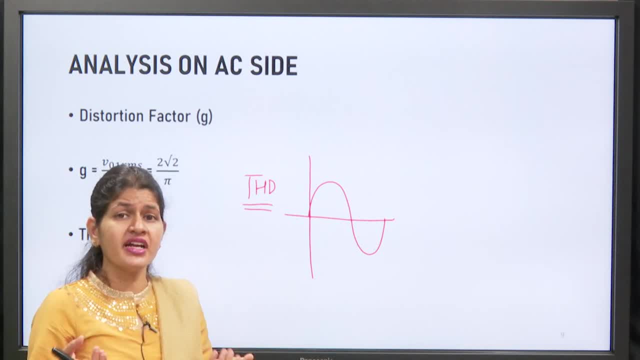 That means how much is the harmonic content in output? This we calculate from THD. So what is the formula of THD Under root 1, upon G square minus 1.. Where this G is. 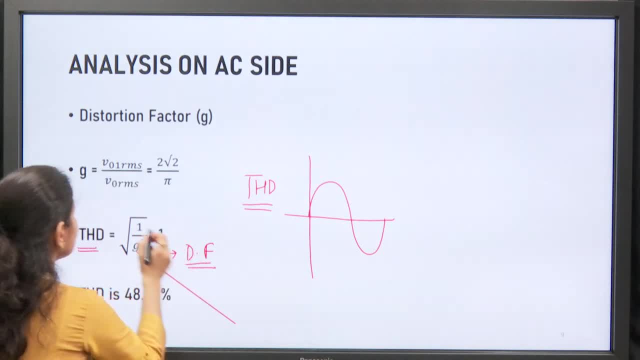 the distortion factor. Right, If we have to find the distortion factor, then what do we do for that V01 RMS which we have found at the back? RMS value of fundamental component upon total output, RMS value. So 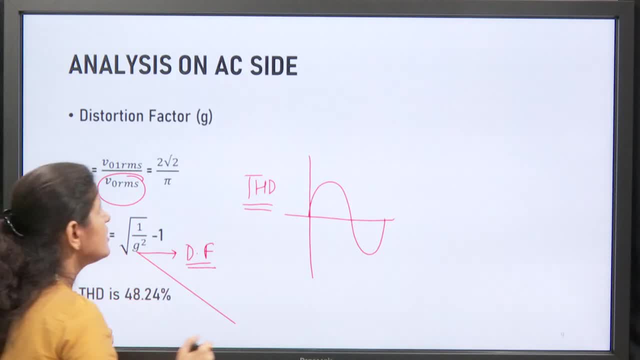 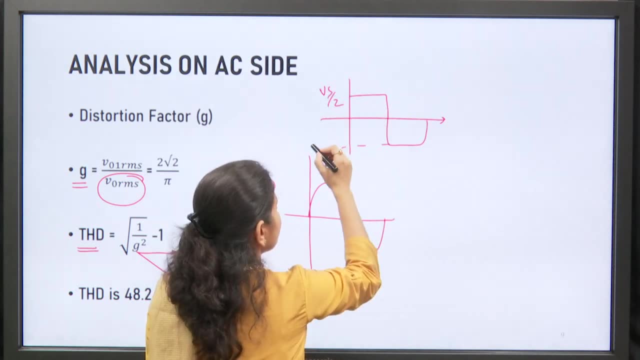 what is the total output we are getting here? Total output, we were getting this Vs by 2, and this is minus Vs by 2.. Right, These two Vs by 2, if we have to find its RMS value, 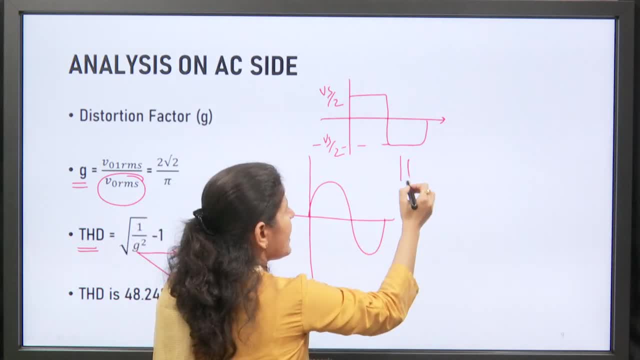 then what is RMS? Root means square, So Vs by 2,. root means square, So first of all, let's do square: Here Vs by 2, and here Vs by 2. So. 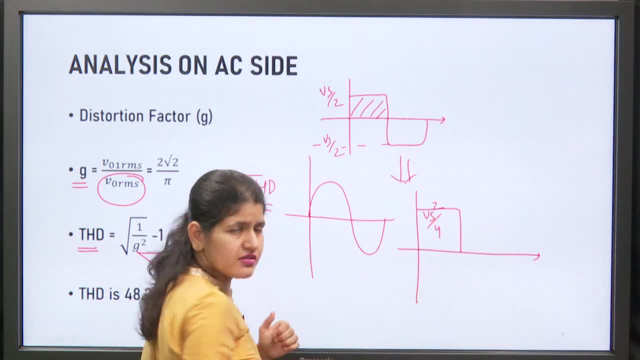 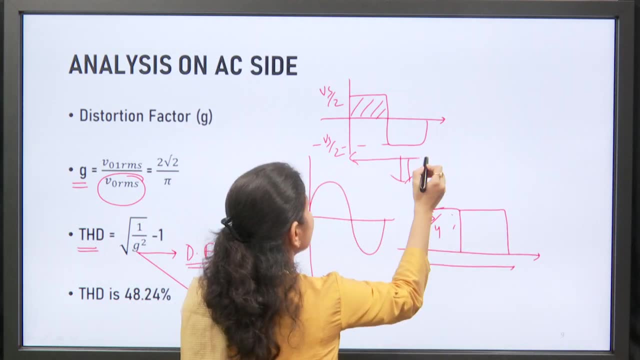 if we do Vs by 2 of this, then how much is it? Vs by 4. Vs, square by 4.. And if we do square of negative part, then how much is it By dropping this line? this: